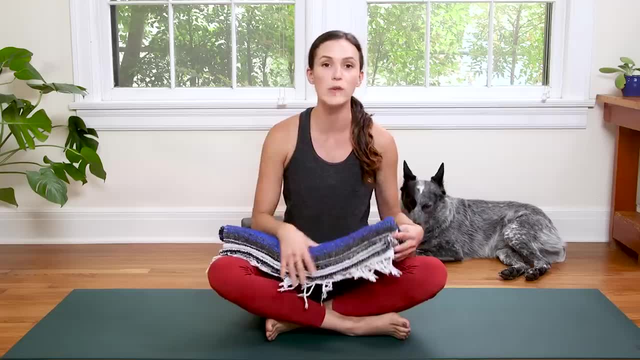 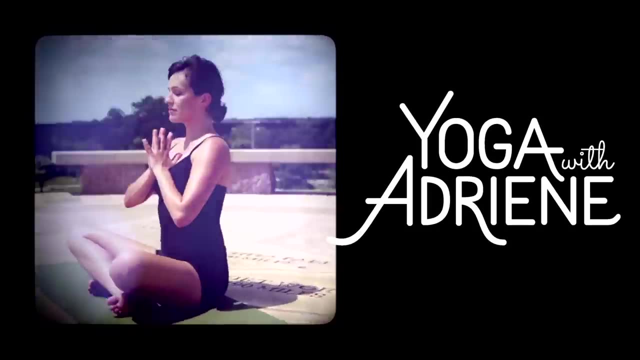 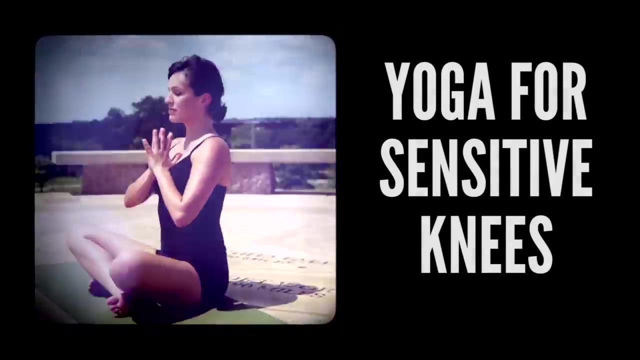 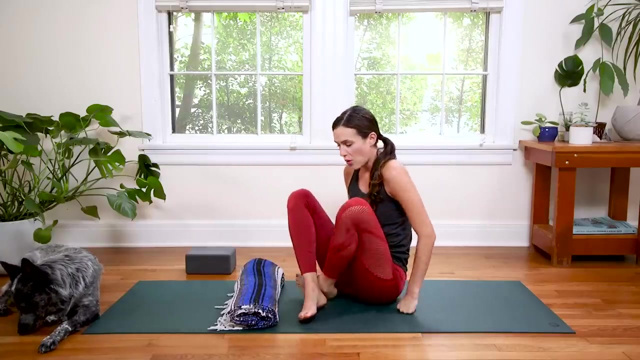 But you don't need it. But everyone's definitely gonna need a blanket today or a rolled up towel. Alright, grab your things and let's get started. Alright, my friends, let's begin seated. We're gonna take our blanket or towel and we're gonna roll it up. 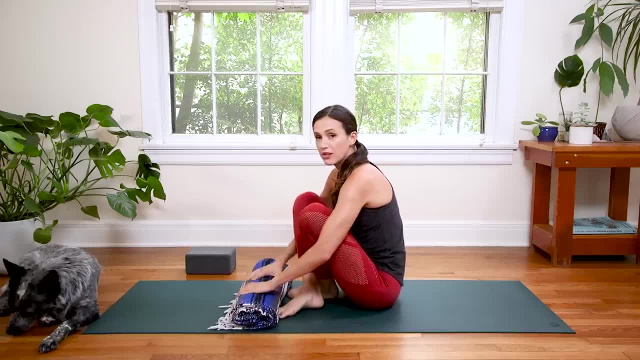 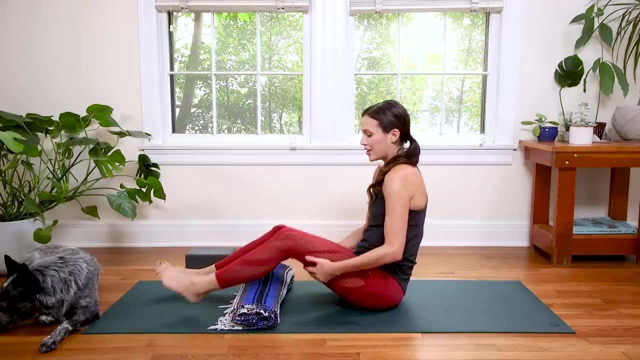 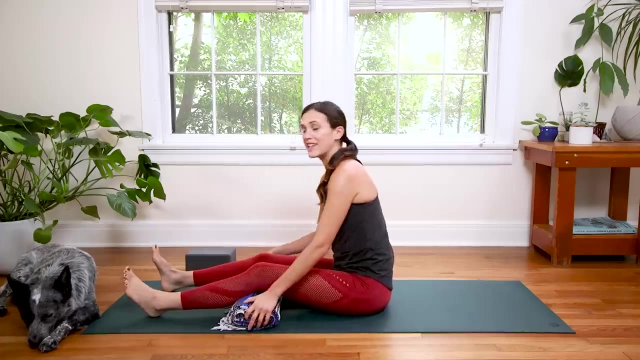 like a little Tootsie Roll. So you're creating a little makeshift at home bolster. If you have a bolster, you can use that, but this really works just fine. You're gonna bring your legs out and you're gonna place that bolster- yep, you guessed it- right behind thy knees. 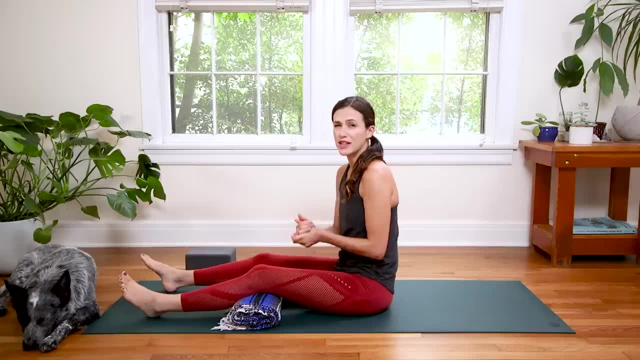 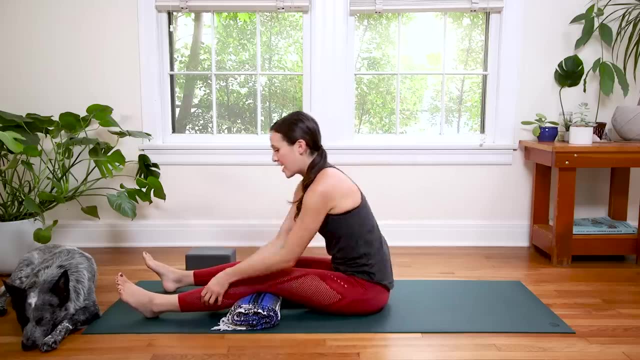 So this is an awesome practice for anyone who just wants to build more awareness in the knees, which I feel like should be could be everyone. So we're gonna start nice and slow and take it easy, Just also kind of using this time as time for yourself to 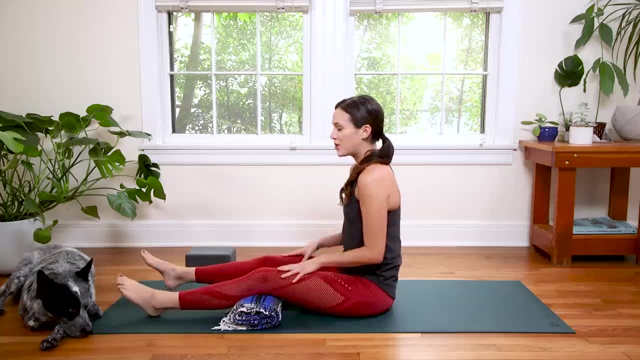 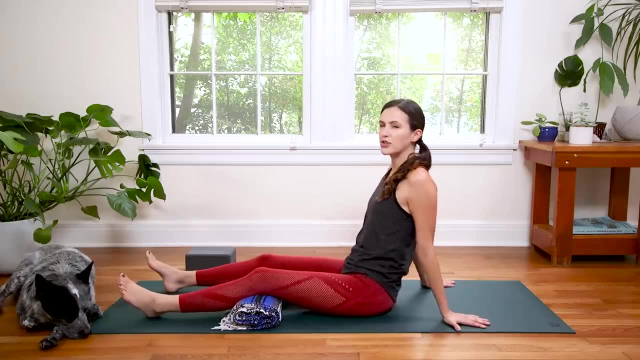 chill out, to restore, to find your breath And bring a little balance to the body. So you're gonna bring your hands to rest behind you in a way that feels good, just so you feel supported and so that you're not collapsed in the spine. 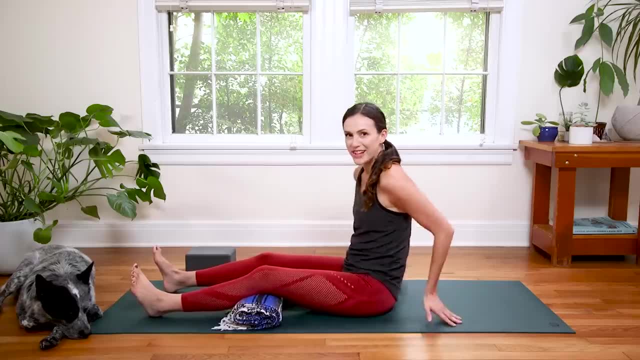 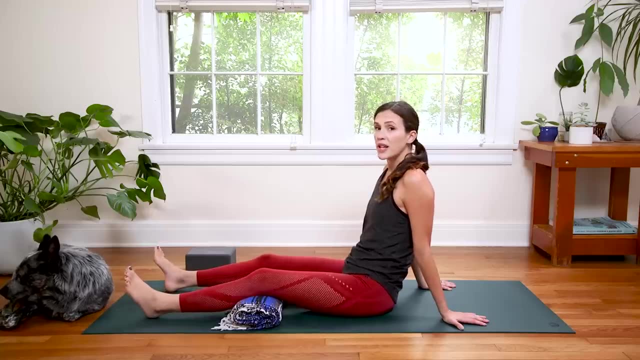 So try to lift up through your heart space Again whichever way in the hands feels awesome for you. Go ahead and find that And then you're gonna take your toes and point them up towards the sky. So there are some things that are just anatomical, right. 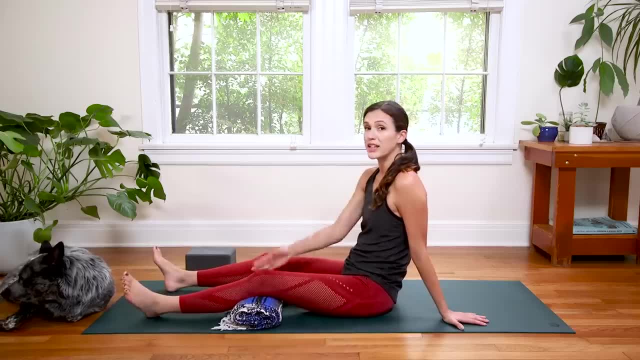 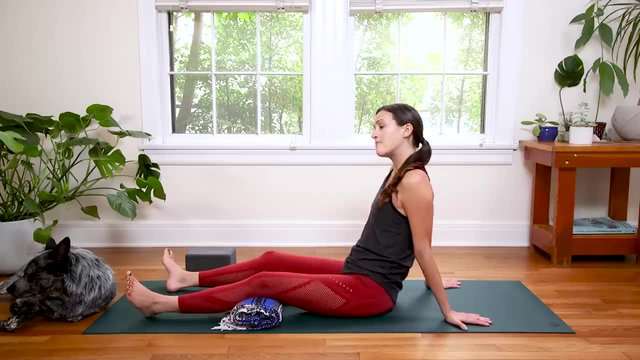 Maybe the toes turn out or the toes turn in, which of course affect the knees. So you walk. So that's all good, But we're just gonna take a little time to experiment and inquire and hopefully bring some stability and strength to the knees without hurting your knees. 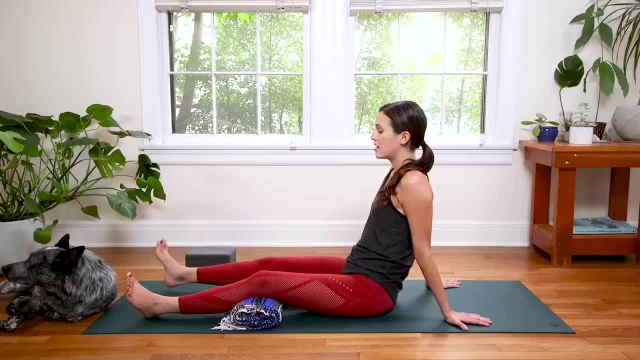 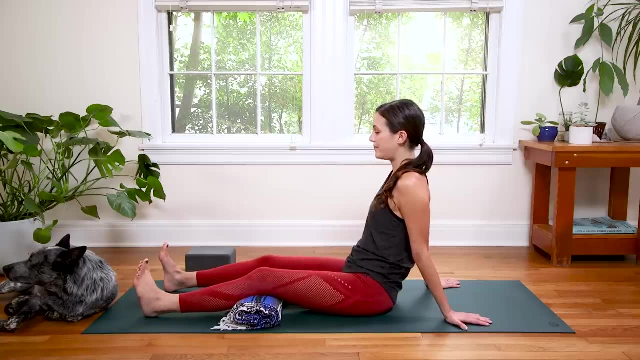 So a lot of people can't do a lot of the at home yoga practices because there's a lot of pressure on the knees. So I got you. Here we go. Bring the toes up towards the sky. Excuse my voice today, Austin allergies. 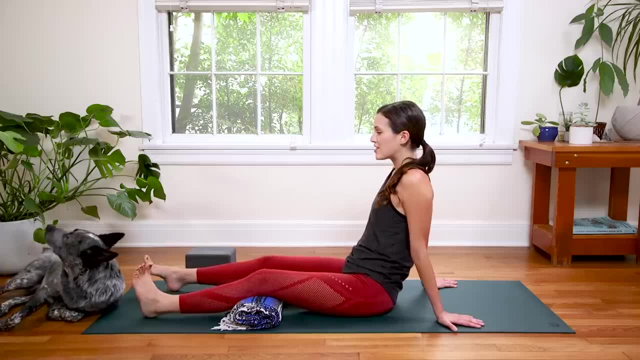 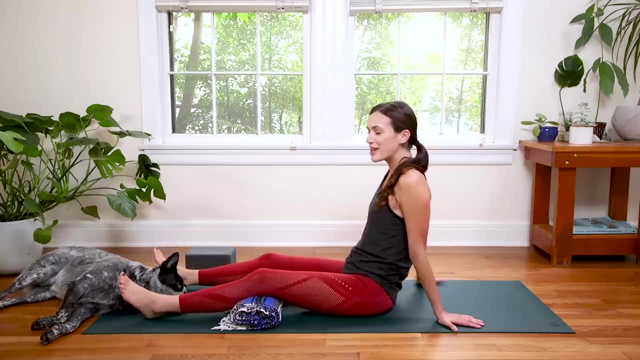 Plus, you know my voice, It doesn't fluctuate. So, hey, buddy, And then bring your toes to pet your dog like so. Okay, no, Gosh, he has to make it all about him. Okay, toes are pointing up. 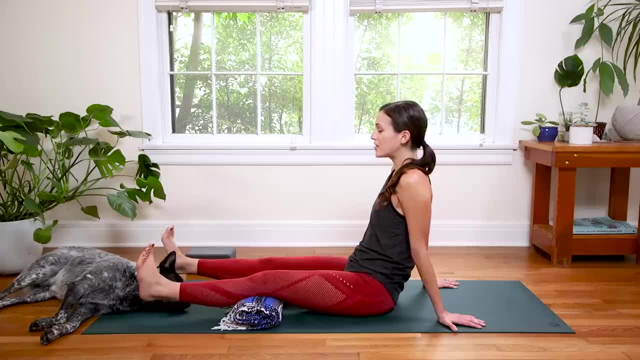 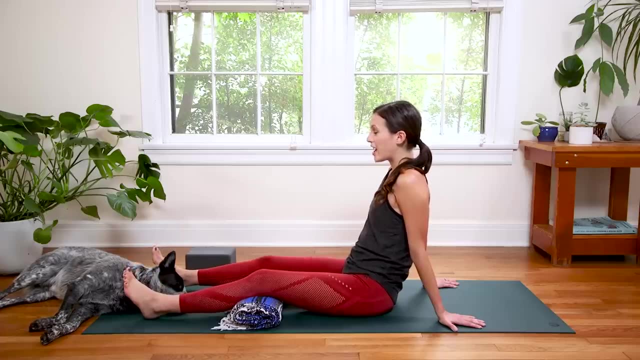 You're gonna lift the heels, I'll focus And as you lift the heels, I just want you to keep a little bit of awareness in the knees. Just notice what it feels like and then lower, And then lift the heels And lower. 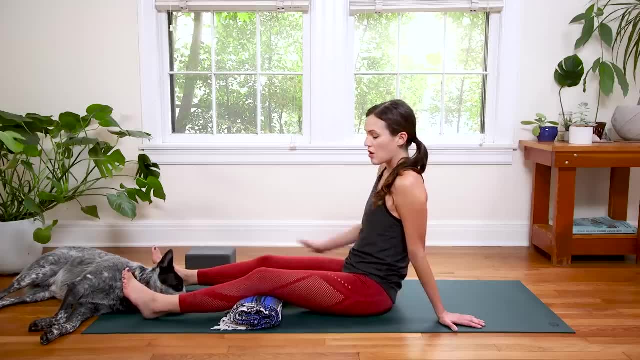 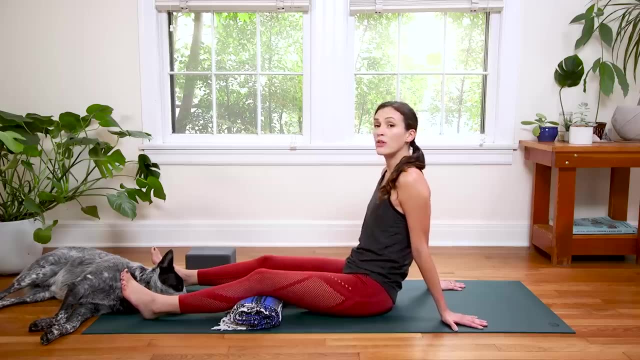 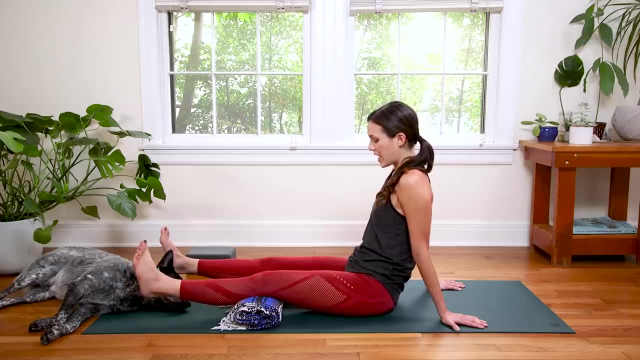 And now, this time, when you lift the heels, notice what muscles around this area- thigh bone, quadricep, inner thigh, inner groin- notice what muscles, if anything turn on Ready, Here we go, Lift the heels, Toes are pointing up. 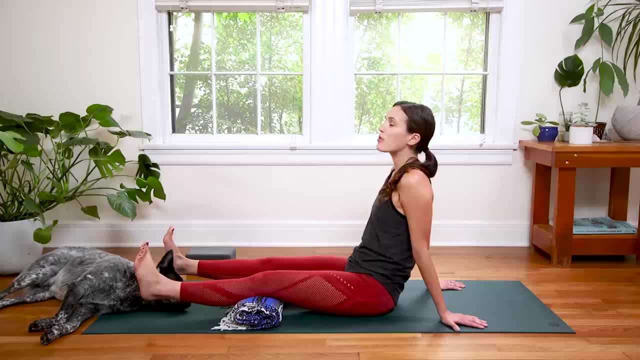 And then if, for whatever reason, you might be clenching in your buttocks right now, relax your butt. Can someone please quote me on that? Relax your butt And then lower the heels. Let's do that one more time. Keep the glutes relaxed. 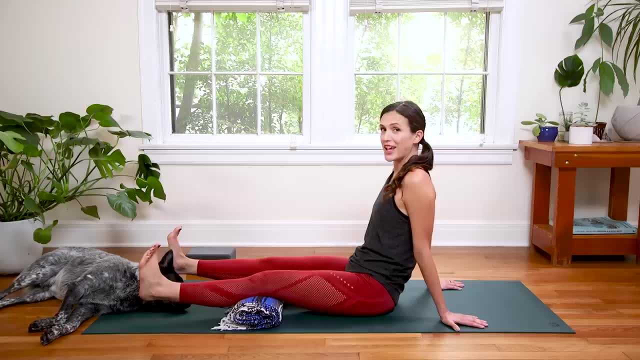 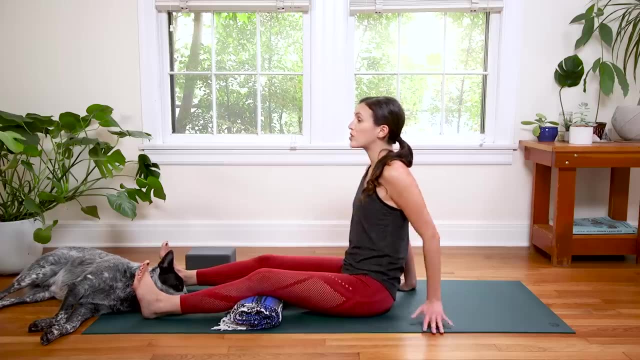 And just notice what muscles turn on. Hey-oh, Alright, Now lower, Awesome. Make an adjustment with the hands if you need to Make sure you're sitting up nice and tall, And then this time we're gonna lift just the right heel and 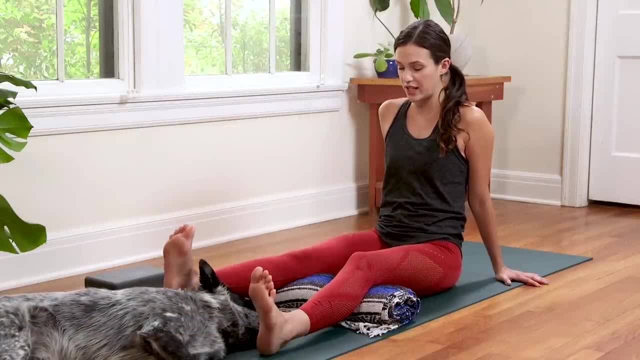 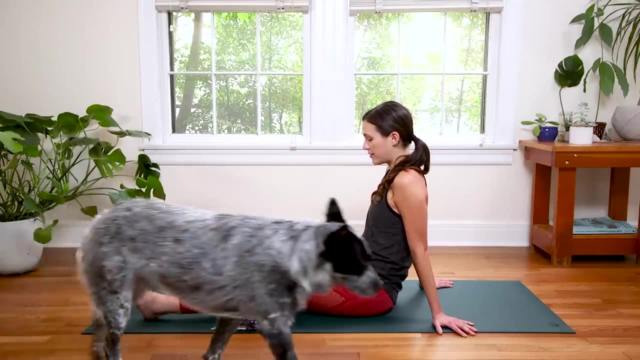 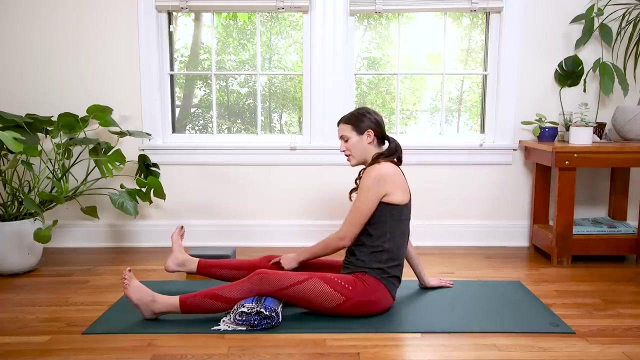 you're just gonna turn the right toes out a little bit and then in Just noticing if we can engage the inner thigh muscle and the quad without clenching the buttocks, And you might feel that in the inner knee- Again, inner thigh. 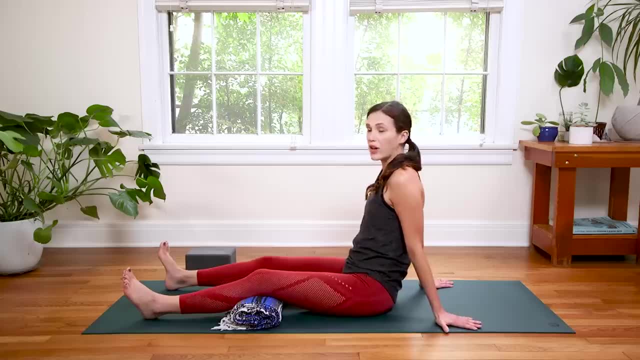 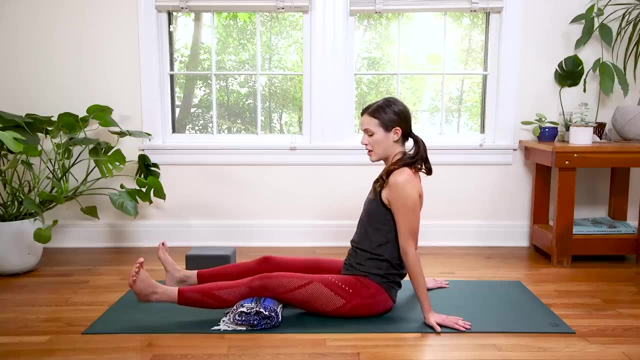 BM And then lower. and let's just try on the other side Again, if your heart is collapsing, see if you can lift up, nice and tall, And then lift the left heel and again nice and slow, So at the very least you're getting a nice little lube of. 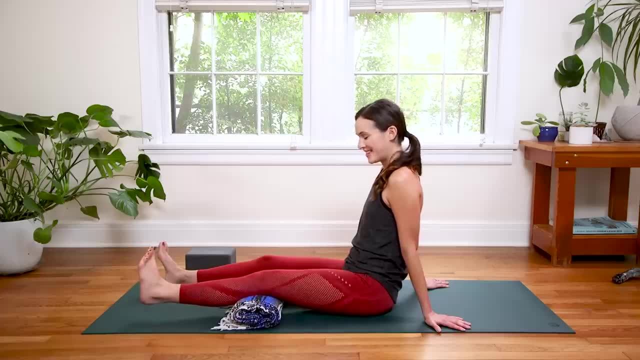 the femur, that hip socket, Okay, And if you take the time to just kind of listen and you can even look down see if, as you turn your toes in and out, you can engage the inner left thigh, naturally you'll engage. 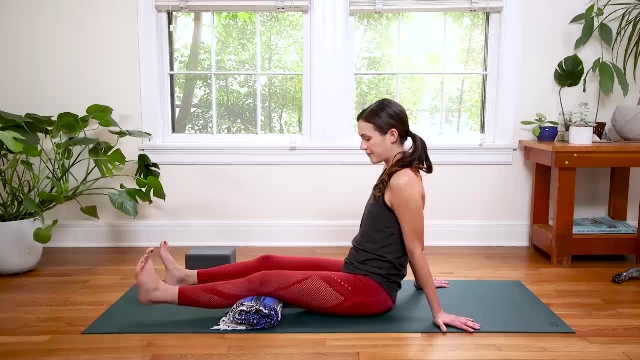 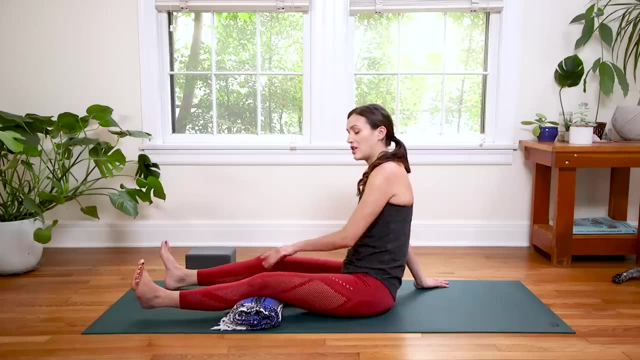 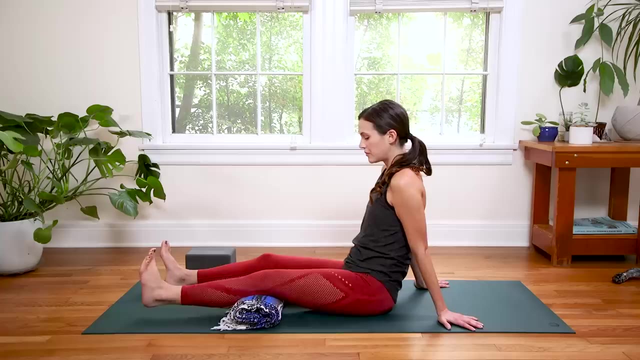 the quadriceps, but without clenching the buttocks, And if you're not used to this, or if you are indeed in need of strengthening and finding stability around the knee, you're going to feel it, maybe in the little inner knee. It shouldn't feel bad, it should just feel like awareness. 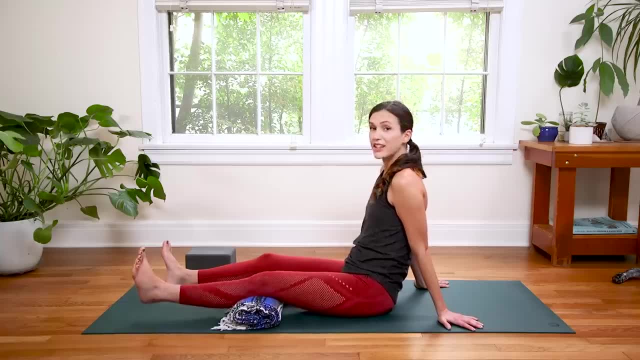 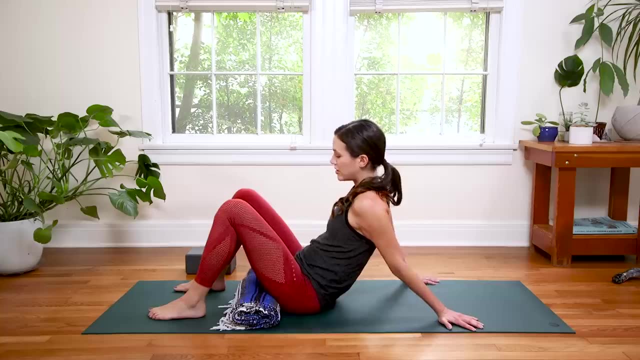 Sweet, And then lower that and then check it out. This is going to be fun. You're going to bring the feet to the ground, bring the butt down to the bolster- your makeshift bolster- and come to lie on your back. Oh yeah. 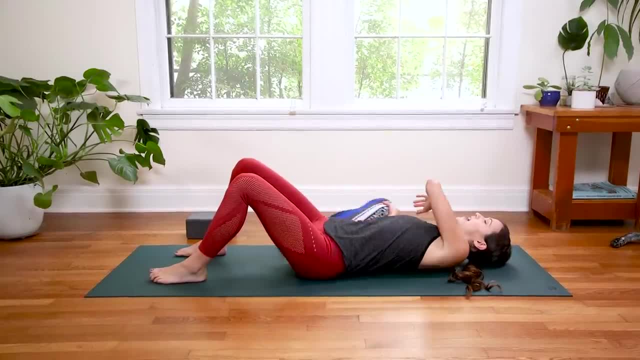 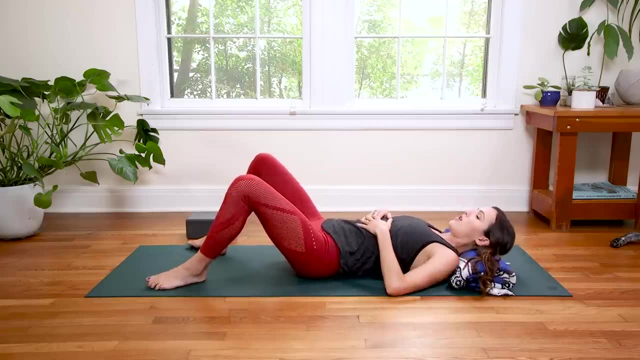 Alright, take the bolster with your right hand, slide your towel or blanket all the way up behind your neck, Yay, And then we're going to slowly walk the feet- excuse me, walk the knees out by bringing the feet together. So, bring the knees out, bring the feet together. 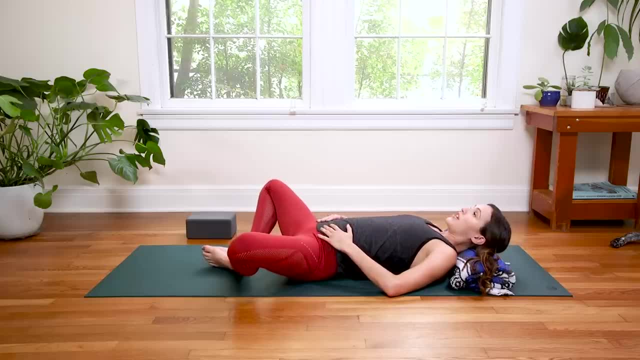 And then bring your hands to your hips and breathe Again, using this time for you to balance the body. Just allow gravity to do the work here. The tops of the thighs nice and heavy, inner groin soft and relaxed. And if you want a little more, you can massage the tops of the hips by pressing palms into. 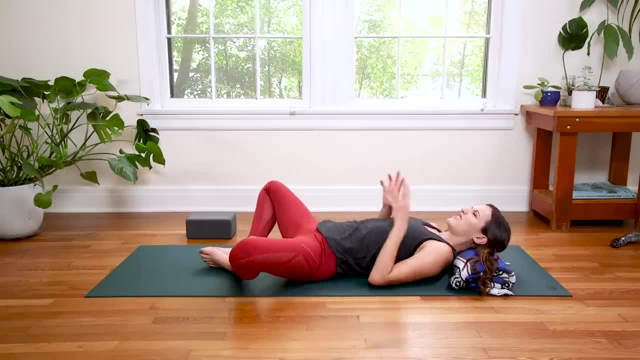 the hip creases. Maybe if you've had some like stress, energy or bad juju you've been carrying around, you can use this to just kind of brush it off, Brush the day away thus far, Start to deepen your breath, Close your eyes. 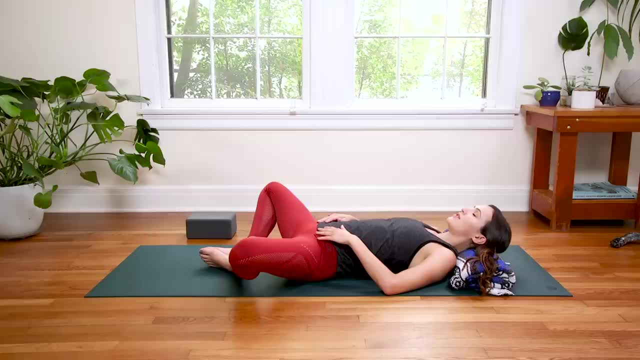 Again. see if you can soften the glutes. Slow, Slow, Slow, Slowly. Take a deep breath in, Let your fingertips, your arms come out, wide palms up towards the sky, And as you exhale, this time, let it out through the mouth a little sigh. 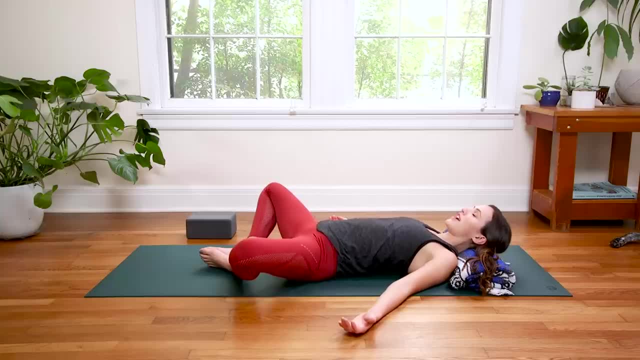 Big inhale in through the nose And again out through the mouth, a little sigh Connecting mind and body. Big inhale And let it go. Cool, Bring the right fingertips to the floor. Good, Bring the right thigh, left fingertips to the left thigh, and you're going to slowly. 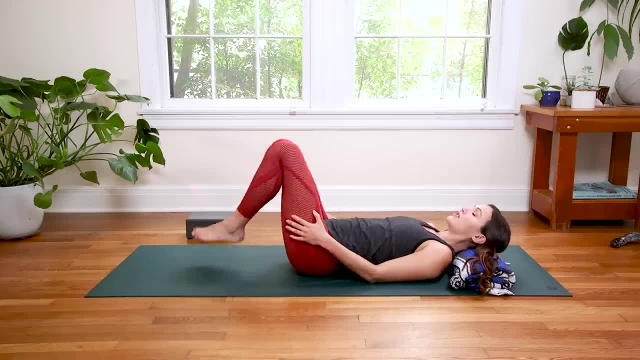 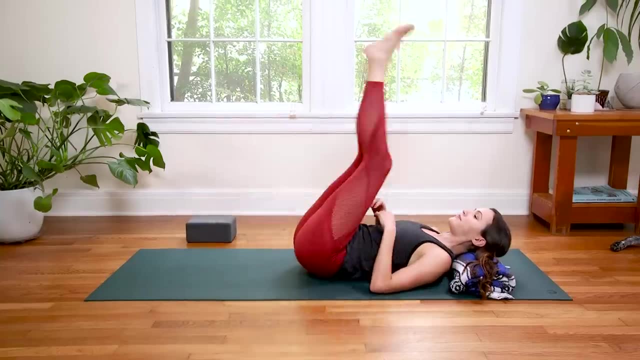 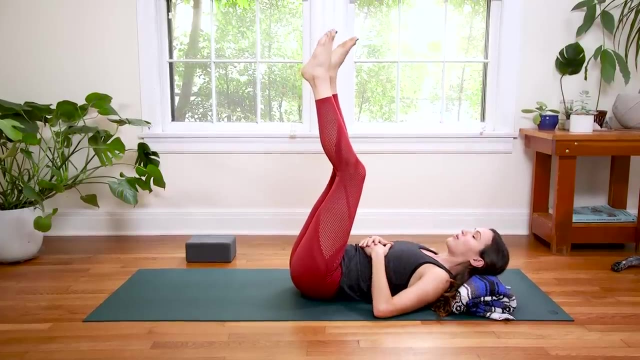 close the legs, Nice, and you're going to send the legs up high, So lower back becomes flush with the mat. so you need a little core strength here, without being on the knees. So none of those cat-cow core strengtheners here, but rather we'll use the support of 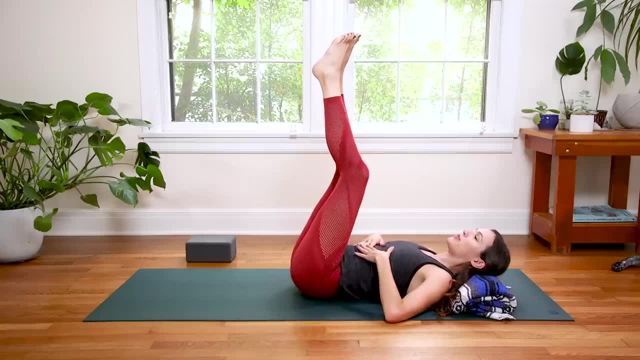 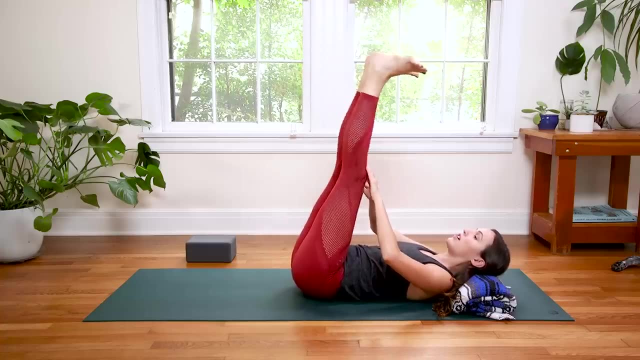 the back. So scoop the tailbone up, engage the abdominal muscles. by hugging the lower ribs in, You can keep a slight bend in the knees. They don't have to be locked. In fact they should never be locked, but they don't have to be straight. 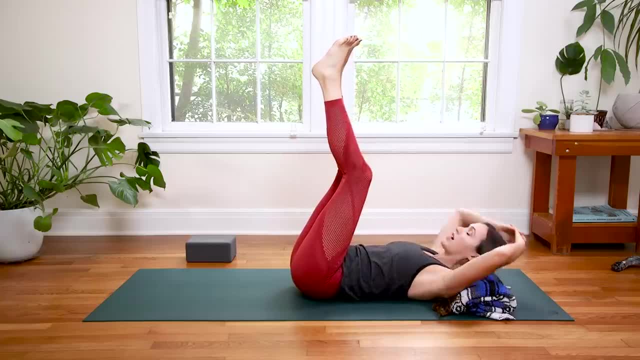 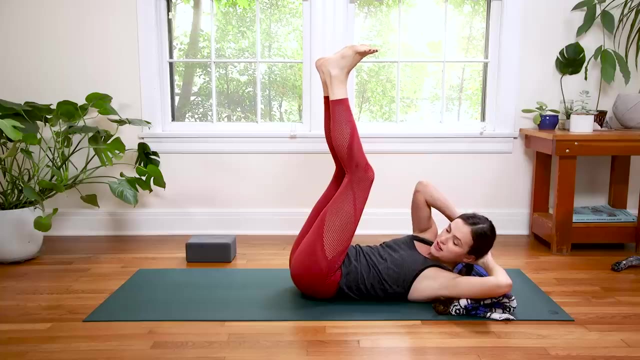 Awesome. And then we're going to inhale, interlace the fingertips, bring them behind the head. thumbs, extended Elbows should fit nicely on your towel or blanket. Inhale in And then exhale. You're going to slowly twist the right, bring the right elbow over towards the left knee. 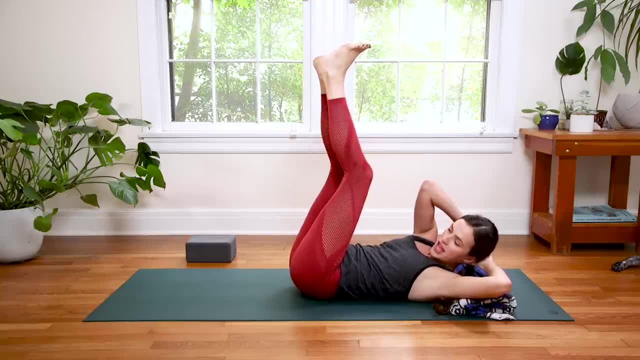 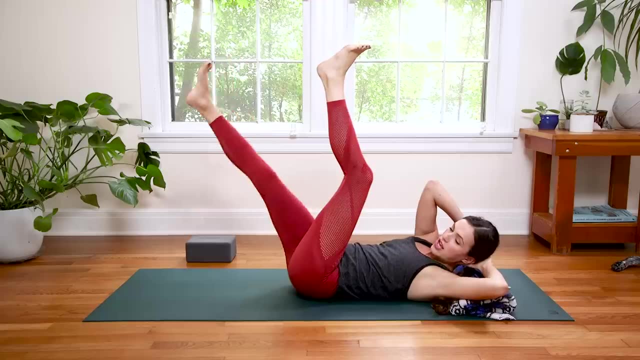 You should feel your abdominals turn on And then you're just going to slowly baby pulse the right leg. Now, if you're able to come down low, you can, but only go as far as you can to where the lower back feels nice and flush with the mat. still. 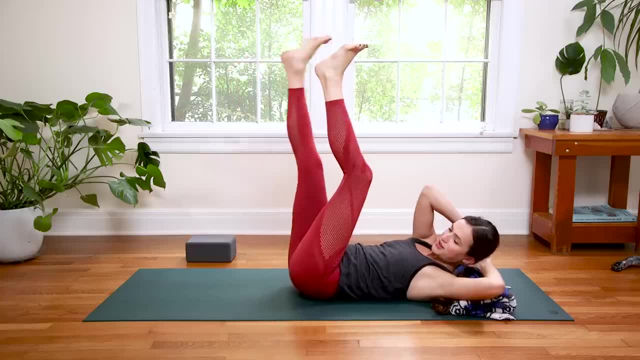 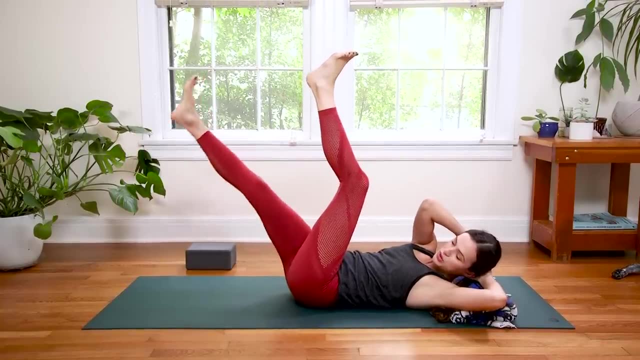 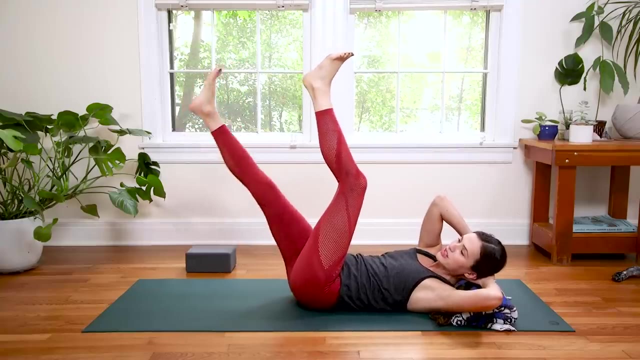 So maybe it's here, Baby pulses. Maybe it's here And you're keeping your twist right elbow reaching towards the front left corner of your mat, Baby pulses And then maybe send your gaze up to not crunch in the neck, Breathe deep here pulsing. 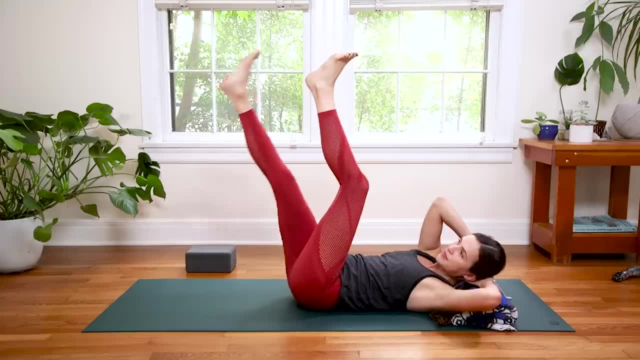 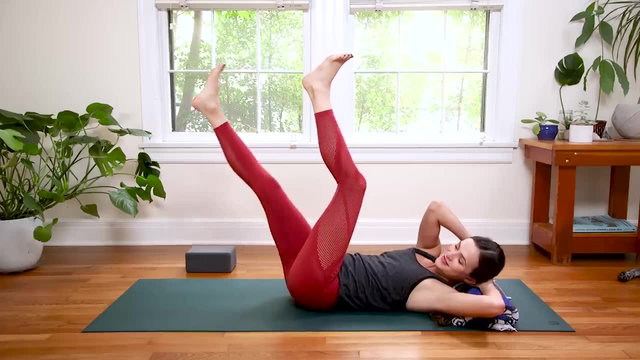 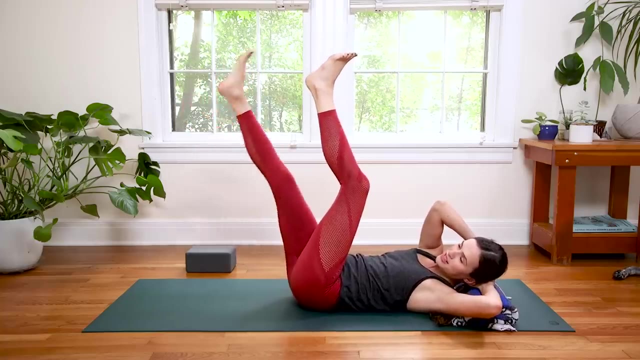 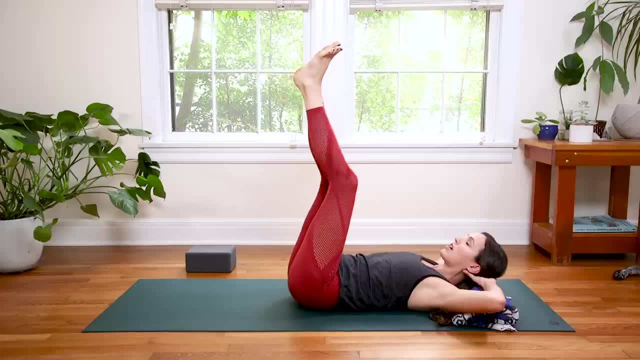 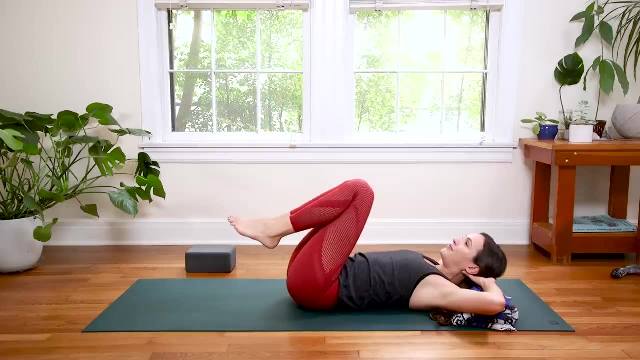 Peaceful in the face. Three, two and then one. Keep the legs up. Feet come together. You rest on your blanket, Take a deep breath in. You can bend the knees here if you need to, And then we'll take it to the other side. 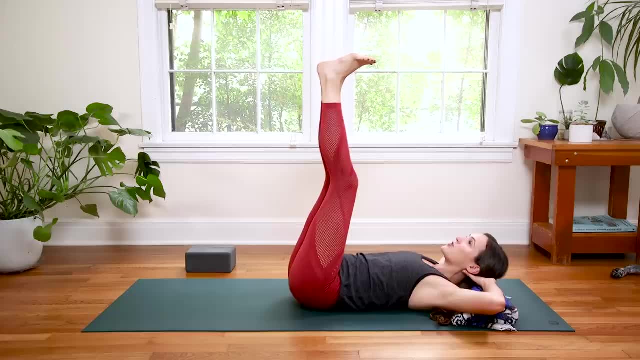 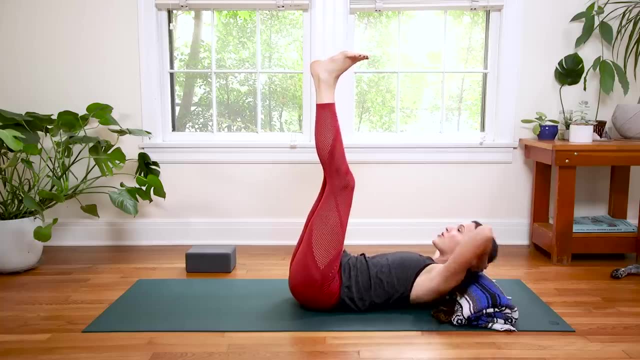 So straighten the legs, Good, Good Inhale. Scoop the tailbone up, Draw the navel down, Hug the lower ribs in So feel that zip up through your abdominal wall And then bring the elbow up and over. 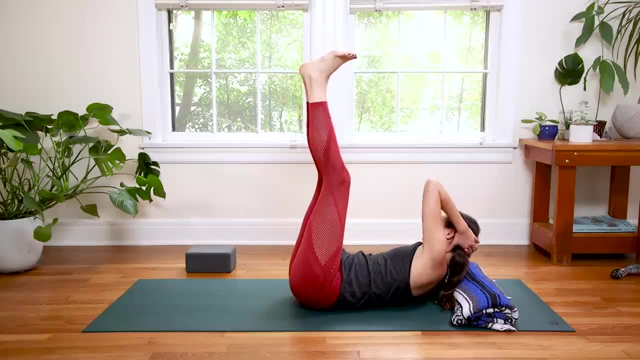 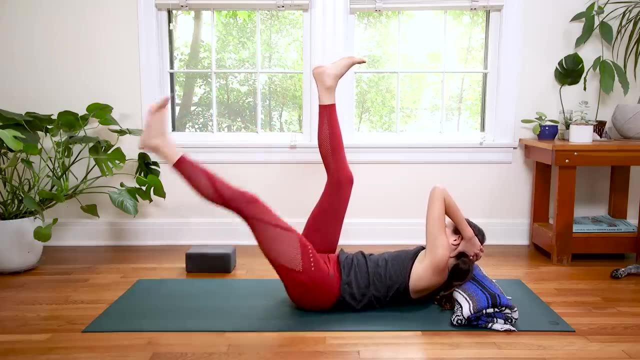 Find your twist. So you're lifting the left shoulder blade up off the earth And then, nice and easy. Listen carefully, Nice, baby pulses again. Extend the left leg. It may not go down as far as you did on the right side. 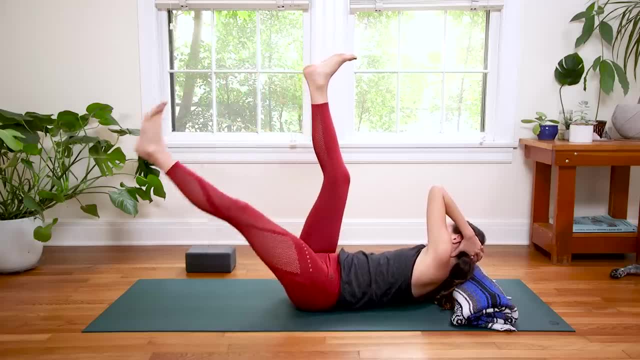 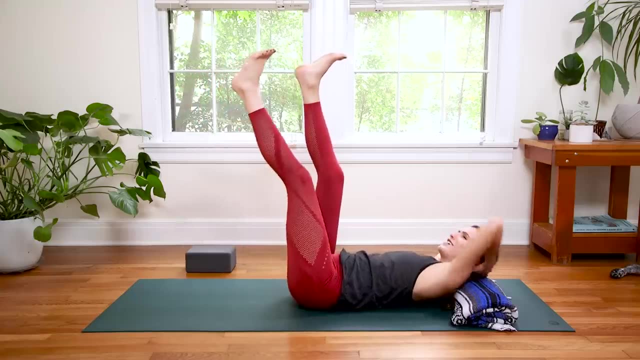 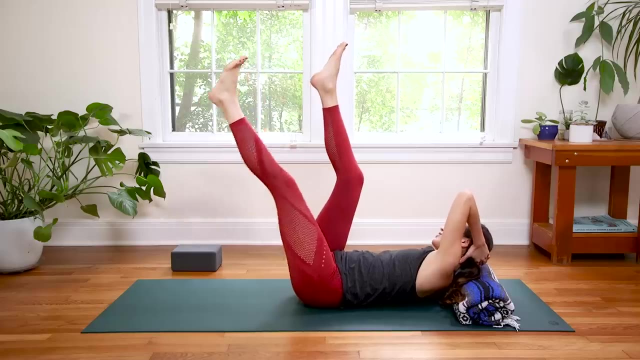 You want to keep the lower back flush Baby pulses. Good, Good, Nice. I did this yesterday, so I'm feeling it Shh, Shh, Shh. All right, you're doing awesome. Gaze up toward that third eye. 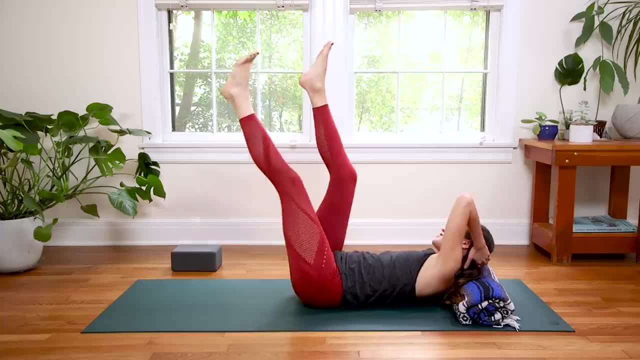 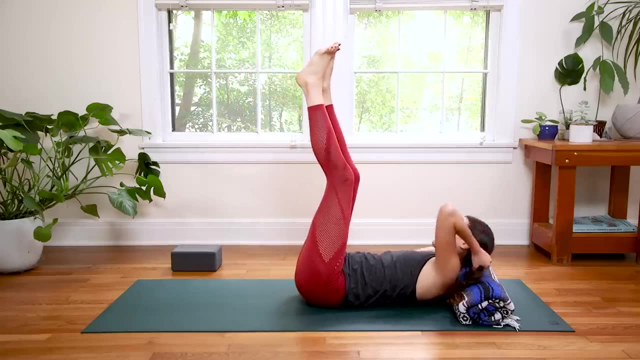 And here we are for Five, For baby pulses. Listen to your breath. Three: Scoop the tailbone up. Two And one: Awesome, Release everything. You're going to bring the hands to the backs of the thighs. You're going to bend the knees. 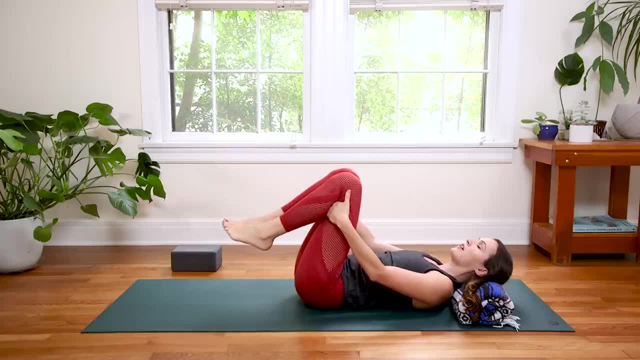 And if you can, And you're just gonna drop the heels down. So lots of different levels of sensitivity here. Some people will be able to draw the knees all the way up to the chest, but your hands are gonna be behind the knees, so there's spaciousness there. 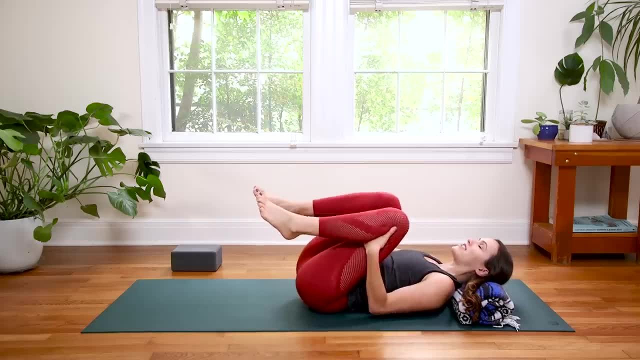 So squeeze the knees into the chest, Scoop the tailbone up. Just feel that last little bit of support on your yoga mat and your back body. Relax your shoulders, Big inhale And then exhale. You can either rock and roll up the length of your spine. 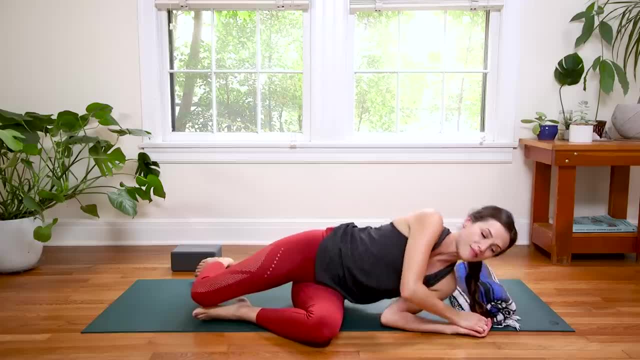 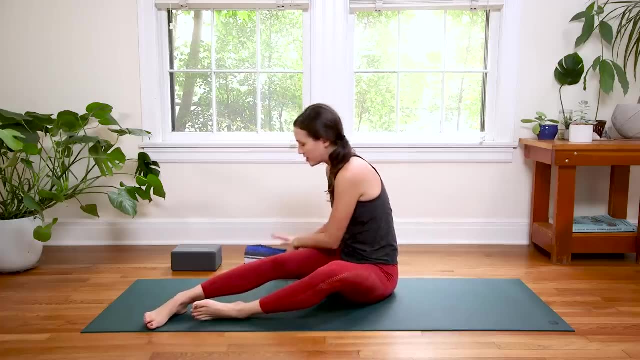 or you're gonna just slowly come to one side And we're gonna come all the way up to a Downward Facing Dog. So take your time. You can put your bolster, your makeshift bolster, keep it rolled up, You can put it to the side. 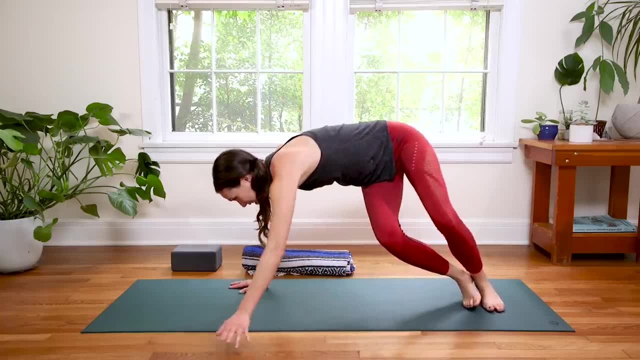 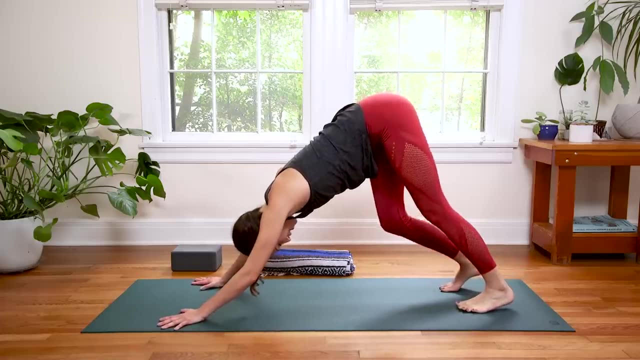 And then we're gonna come all the way to Down. Dog, Keep an awakeness on the live energy in the toes and the feet as you move And then claw through the fingertips when you get there and start to pedal it out. Send the hips up high. 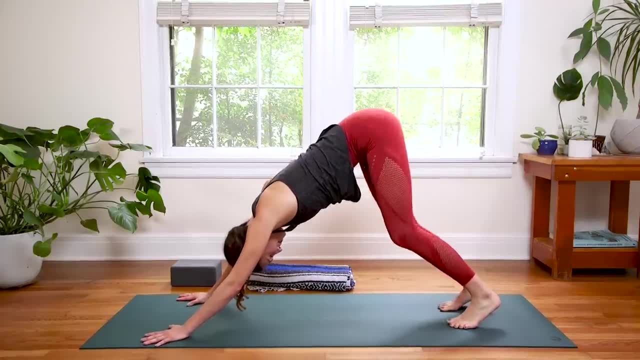 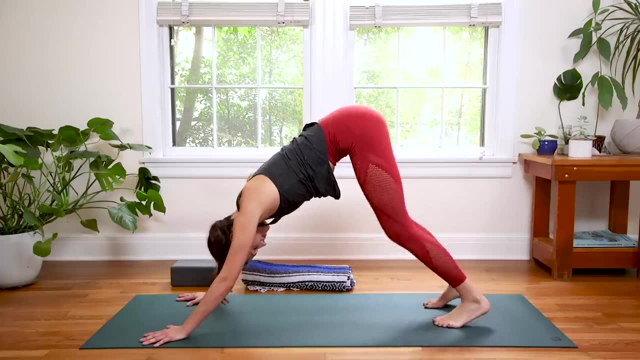 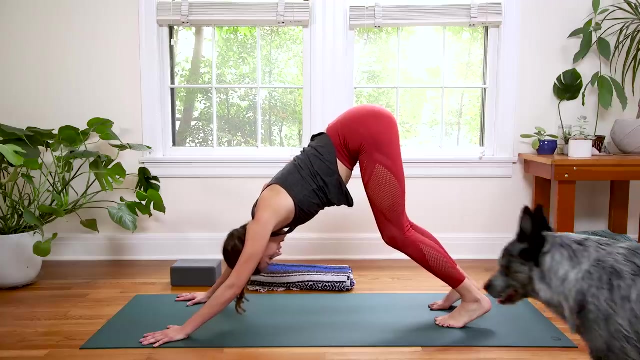 Keep the knees nice and bent. Exhale, Then inhale in deeply. Allergies And then exhale. Melt the heart towards the thighs, Press the heart back, Feel that stretch through the shoulders, the chest Claw through the fingertips. 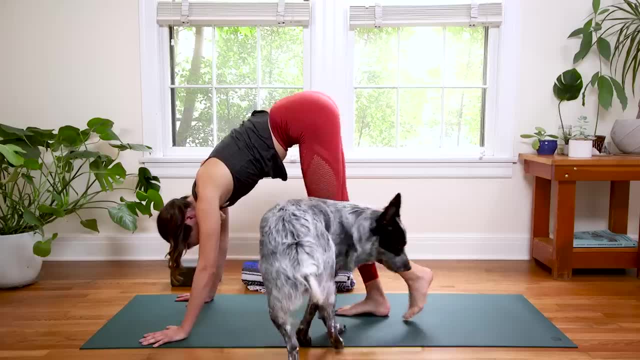 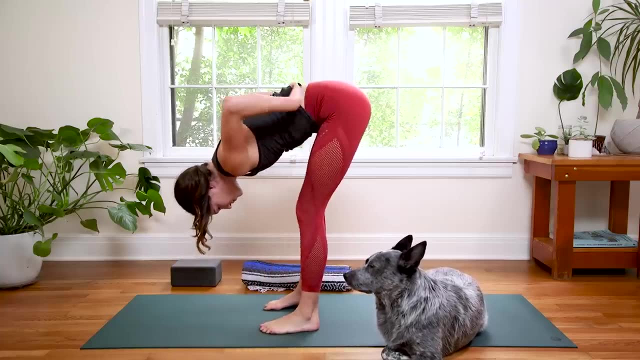 And then slowly you're gonna walk your feet up towards the center of your mat. Nice and slow Feet hip-width apart. You'll come into a little Rag Doll here, a little Forward Fold And again nice slight bend in the knees here. 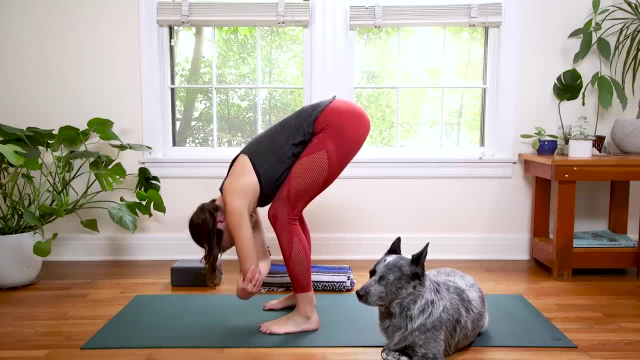 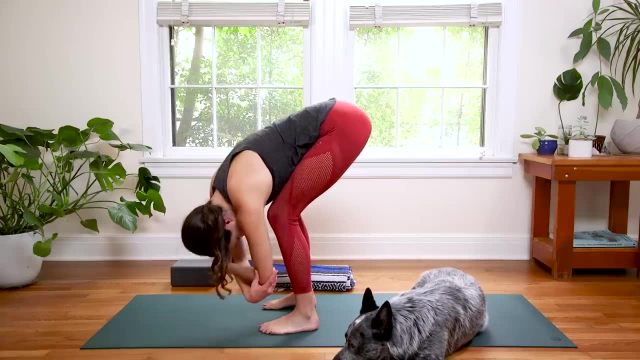 Breathe deep and feel that big stretch in the lower back body as you bend your knees, Connect through your feet all four corners, grab the elbows And you might just rock gently side to side, creating that semi-circle, semi-circle. 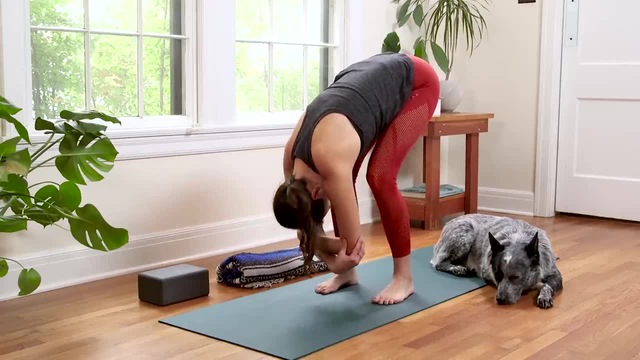 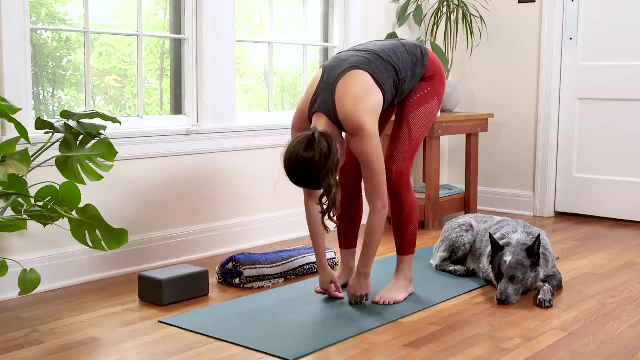 Semi-circle or semi-circle, Semi-circle or semi-circle, Semi-circle, Semi-circle or semi-circle, Semi-circle, Semi-circle, Semi-circle or semi-circle. Take the head loose and then release the arms and slowly press on all four corners of the feet. 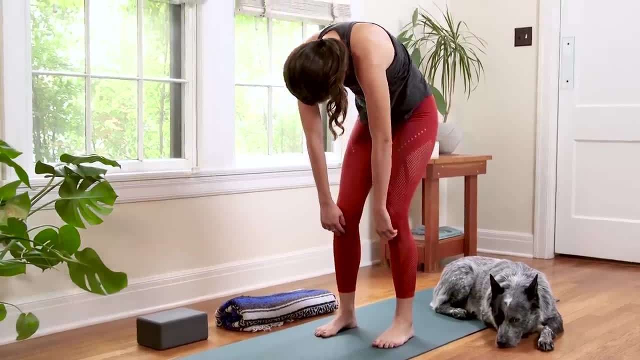 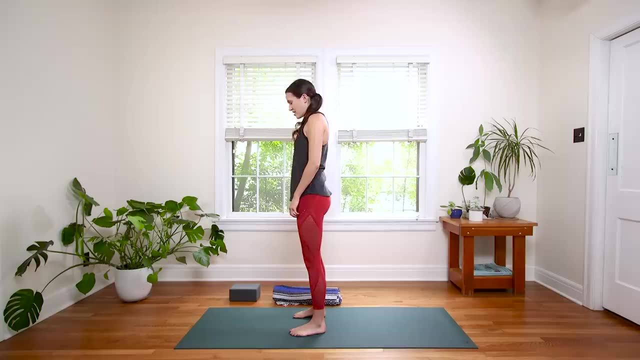 to roll it up And root down through the feet as you rise up, lift the chest, lift the sternum and right away you're gonna bring the fingertips around, interlace behind your back and draw the knuckles down and away. open the chest, breathe deep. 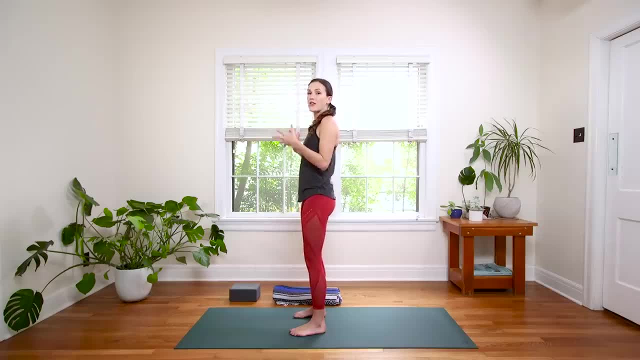 feel this upward current of energy through the front body and allow your body to respond to that. So if the pelvis is dipping out here and you're thinking upward through the front body, bring your hip points all the way up towards the sky. Just kind of bring your center underneath you. 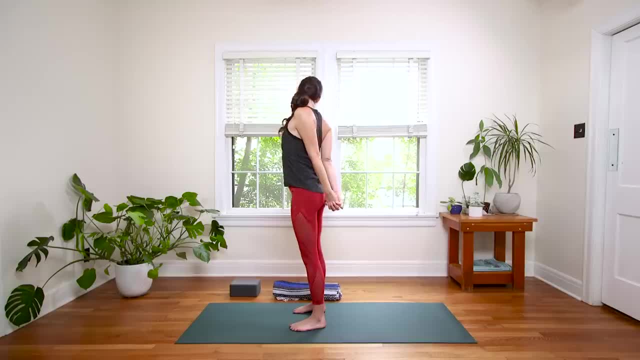 And then you might open the throat a little bit. here You might find soft, easy movement that feels awesome. Take a deep breath in and then exhale. bend the knees and take your knuckles, draw a big rainbow So they actively reach up towards the sky. 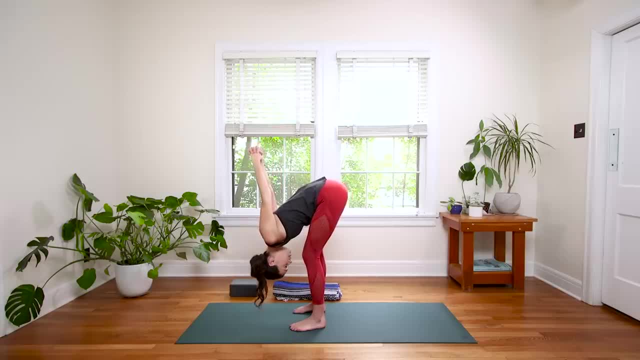 all the way up and over. Big stretch requires big breath, big inhale, Then exhale all the way back up. Great, then you're gonna cross the right arm over the left, over the body. give yourself a big hug, Inhale, root down through the feet. 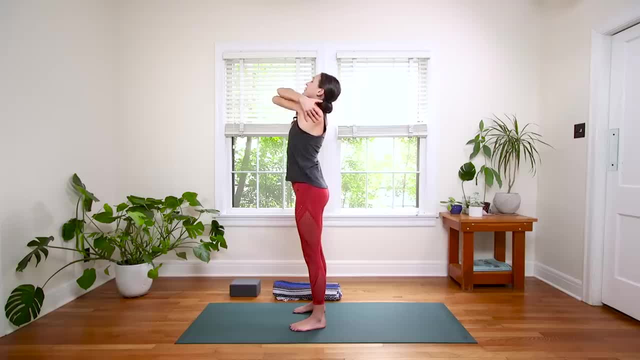 lift up through the inner thigh here And then exhale, release, Interlace the fingertips behind, this time opposite thumb on top, so reverse your grip and then draw the knuckles down and away again. Inhale, lift the chest, lift the throat. 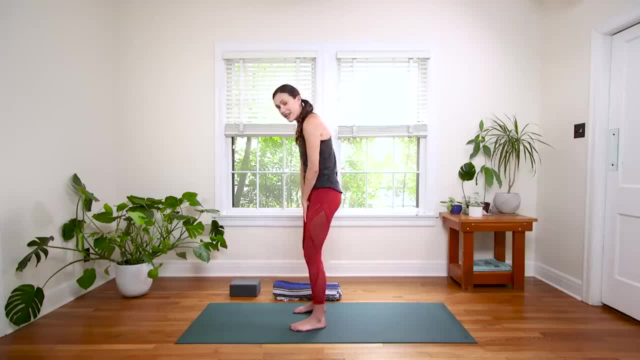 and draw your center underneath you hip points towards the sky. This is gonna require that inner thigh and the quad to kind of turn on again. See if you can locate that. just play, Maybe lift the toes on this one, And then here we go bending the knees. 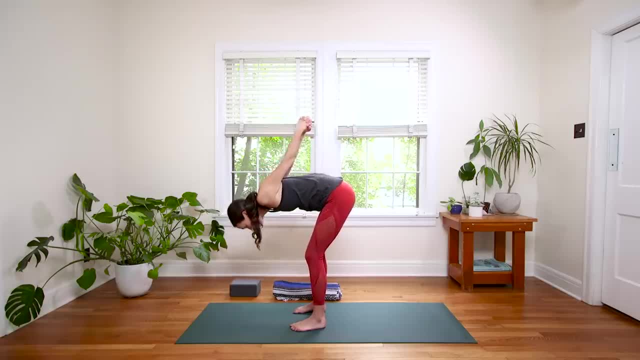 bringing the heart forward first and then down knuckles. draw up towards the sky, Big stretch, so big. inhale to support And then exhale to press into the heels. draw the knuckles back. heart lifts up. Release your grip. feel that flush of energy. 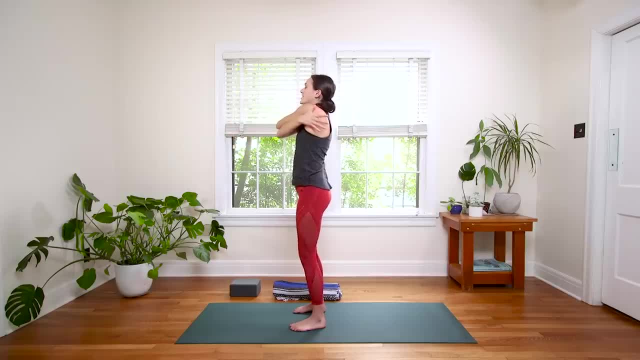 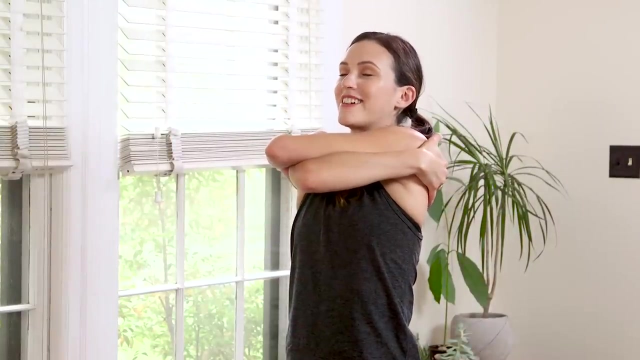 and this time big hug, left arm over the right And take a second here to draw up through the arches of the feet. So again feel that inner thigh lift, but also to just feel this embrace, feel this hug, Feel the expansion in the lungs. 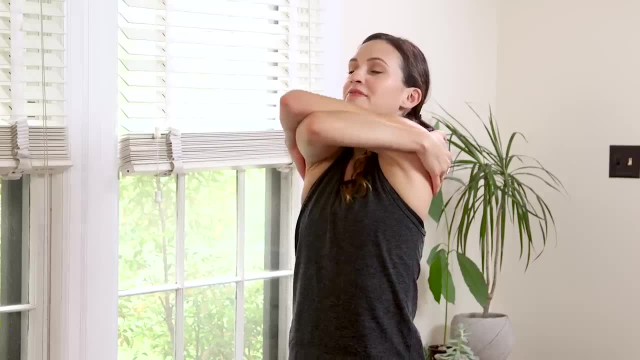 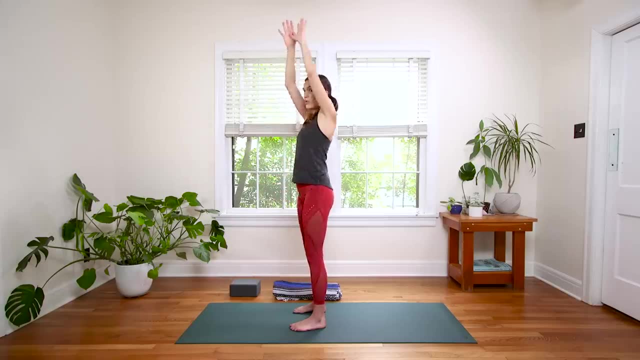 the upper back body and the ribs as you breathe in And then exhale, release it out. Awesome inhale, send the fingertips up high this time. Wu-Tang grip today. big inhale as you hook the thumbs, fingertips reach up high. 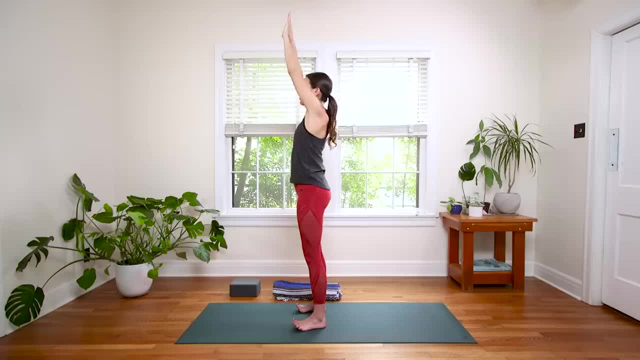 And then exhale. keep lifting up through your arches, So press in all four corners of the feet, especially the outer edges. So if you tend to roll in towards the inner arches, press to the outer edges And then, as if you were in between two panes of glass. 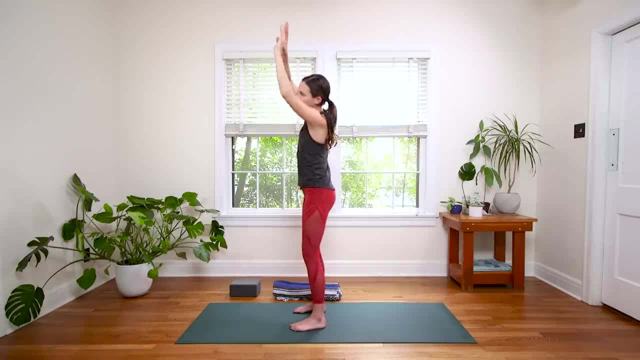 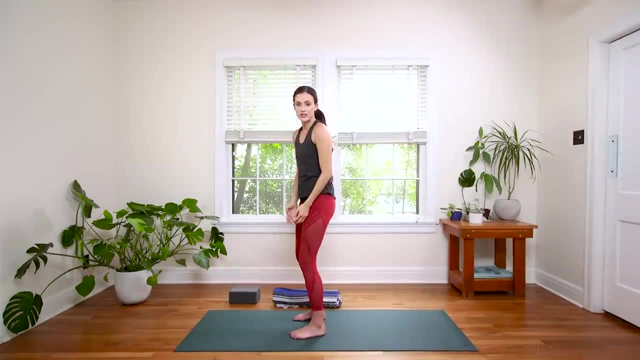 just slowly tilt to the left, So not a big bump, but just a slow tilt, And then lift up from your pelvic floor. And a lot of times in yoga you'll hear someone say: lift up from your pelvic floor. And a lot of times in yoga you'll hear someone say: 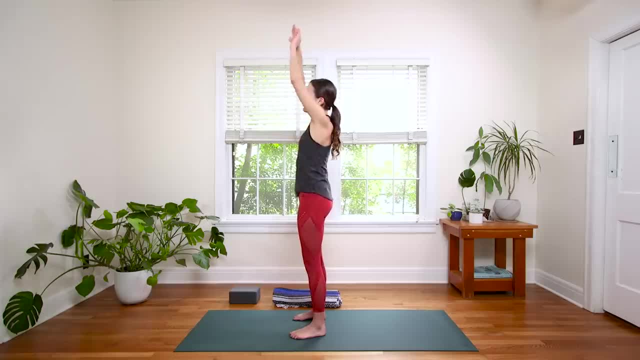 lift up from your pelvic floor And a lot of times in yoga you'll hear someone say: lift the kneecaps. Think about engaging the inner thighs and the quads without clenching your glutes And then back up through center, press through the feet. 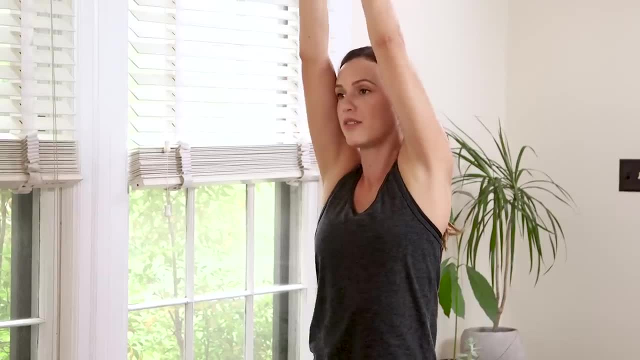 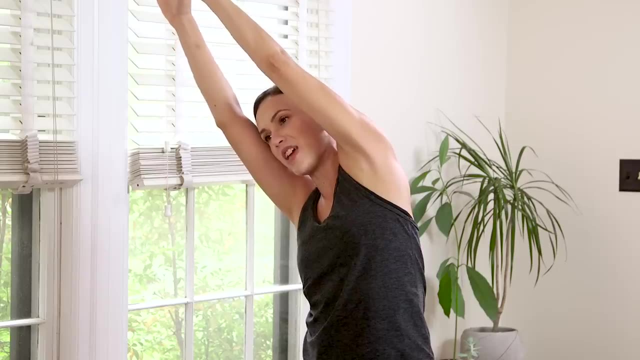 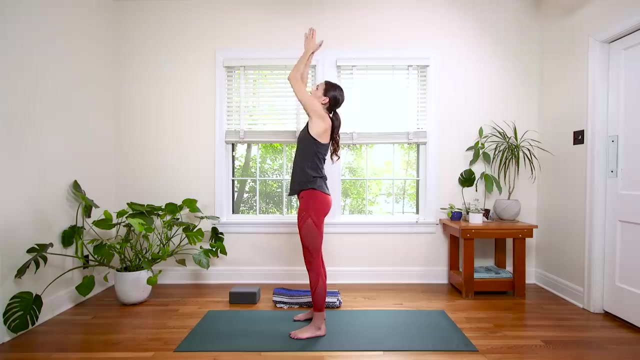 reestablish your foundation ground through the feet and then slowly, sliding to the other side, Tuck the chin slightly, See if you can lift up through the inner thigh, just a sensation- And then slowly bring it back. Palms come together and down at the heart as you. 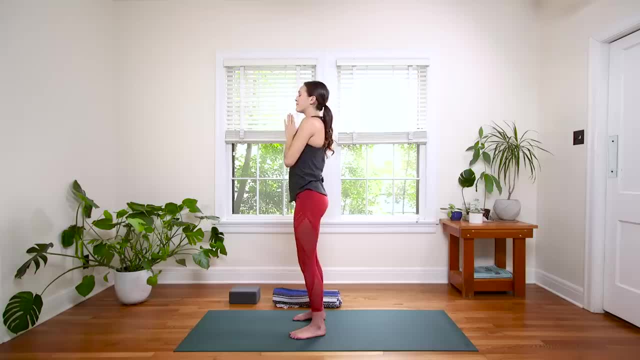 breathe out. Anjali Mudra: Awesome. deep breath in, Long breath out. Now resist the urge to look down. You can, of course you're the boss, But keep the palms pressing together and this time bring the elbows out. 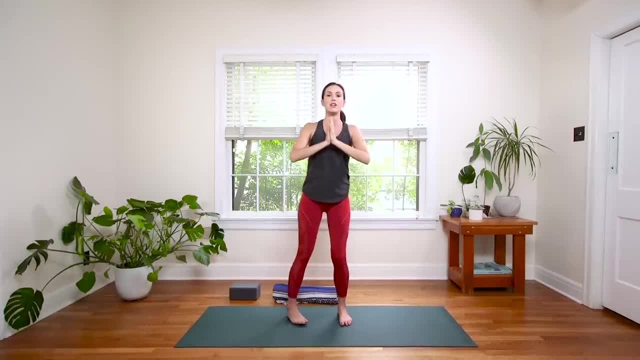 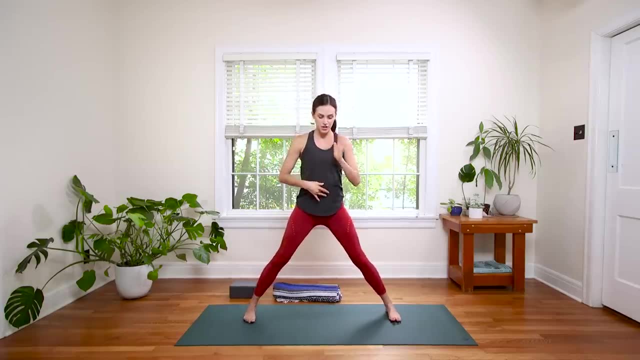 And then just trust that the earth is there. and if you don't wanna step out wide, you can keep the feet on the ground and slowly move your foot out. We're just gonna step out nice and wide. Stay connected to your core for stability. 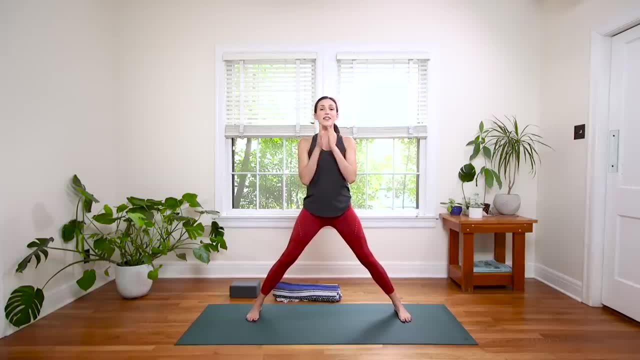 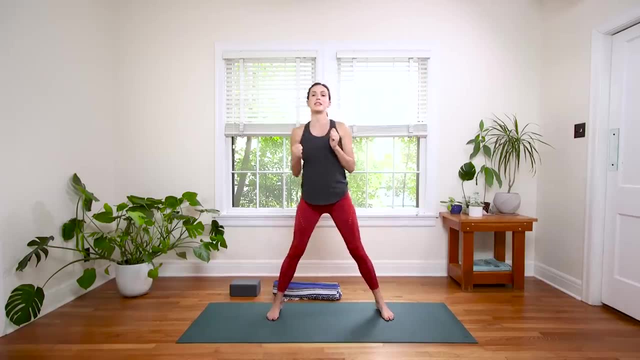 It's hard not to look down And then turn your toes just so they're facing forward. so feet are nice and parallel And if you're feeling any pressure on the knees here, bring your stance in weigh in, Otherwise we'll lock it out. 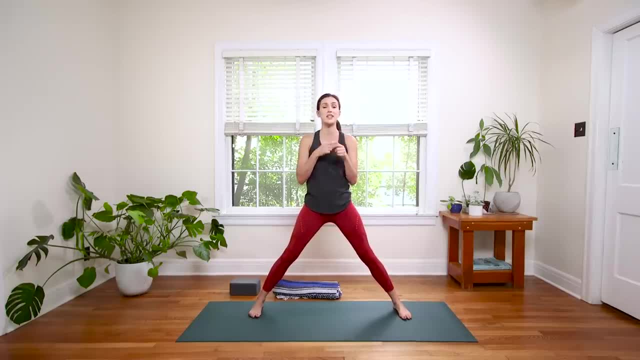 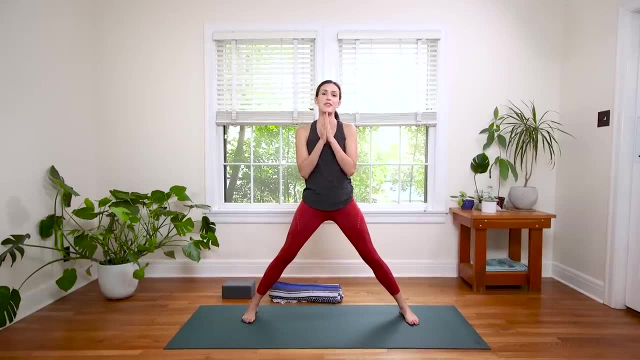 Alright, so I'm giving us time to set these up, because a lot of times what happens with the knees is we just get rushed into doing something in a public class or even at home, or we just haven't trained our mind to consider the nuance of things. 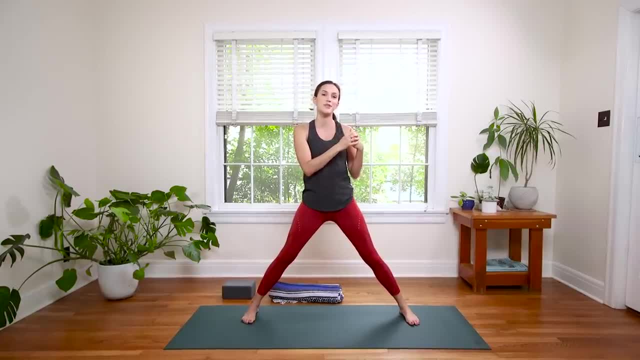 and we're just setting ourself. we're not setting ourselves up, So we're. there's a lacking of setting ourself up for a strong foundation in the posture, which can put a lot of pressure on the joints And if you're dealing with an injury. 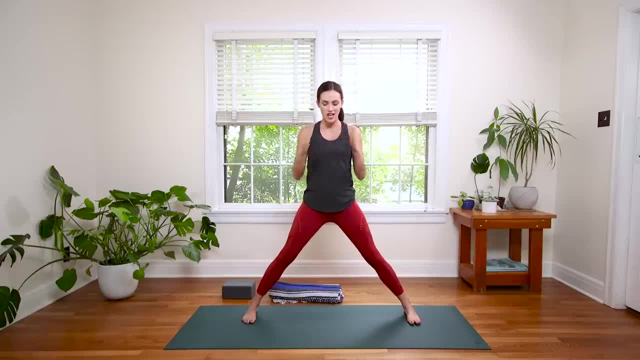 or something in healing. forget about it. So take your time. Toes are pointing forward. Lift up from the arches of the feet. Engage the inner thigh in the quad that we did when we were doing that little beginning exercise. Lengthen tailbone down without clenching the glutes. 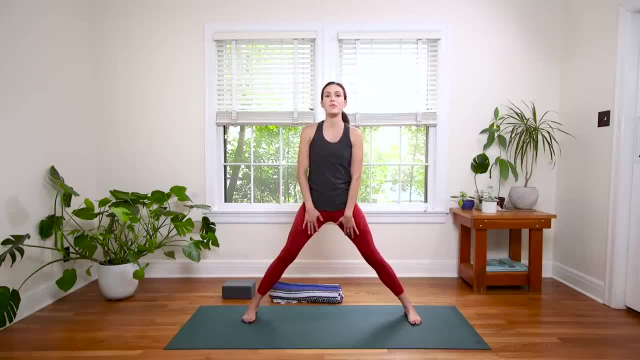 So it's not just a tightness and a gripping, We're activating hugging muscle to bone With awareness. So lengthen tailbone down, Just play with that here. Not so much here, but right here, And then hands come back to the heart. 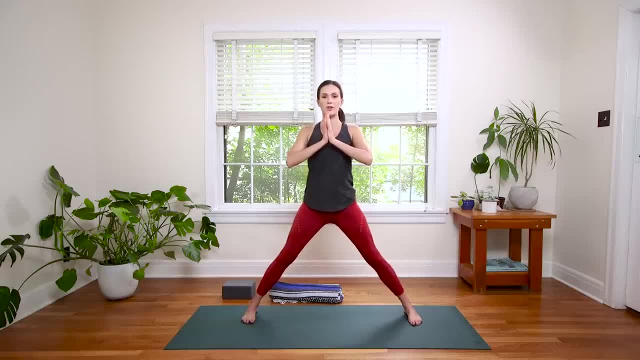 Elbows out wide whenever you are ready, Or maybe you're already there. So again, think up. We're kind of zipping up from the arches, We're lifting up from the inner thighs, inner groins, And we'll continue that motion from the lower body. 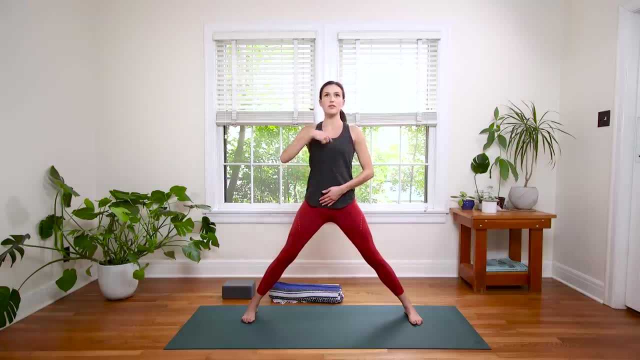 all the way up through the spine. So lift up through the pelvic floor. Imagine it rising, rising, rising all the way to the crown Shoulders. nice and long spine. lengthened Inhale in, Exhale, slight bend in the knees. 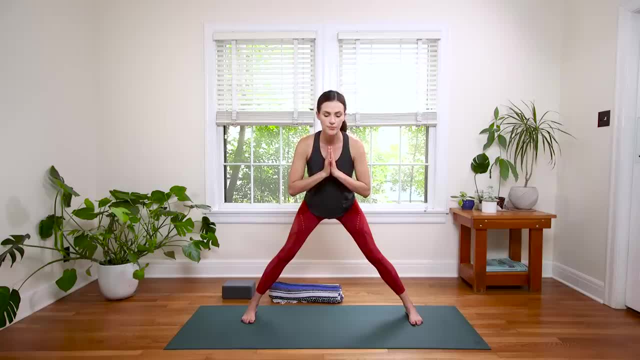 Claw through the outer edges of the feet and slowly just send your heart forward And then come back. However far you made, it is good. Inhale in again and exhale. draw the navel in, Connect to your center, your core stability. 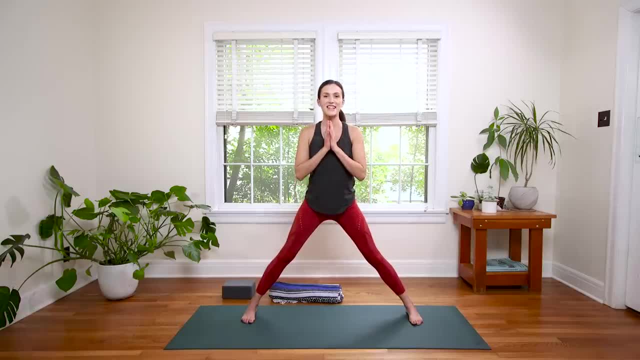 and come forward, Oh yeah, And then come back. And then one more time. Maybe you go a little further and maybe not. Listen to your body. Draw the navel in and up. Maybe you come all the way down. We're here for three breaths, wherever you are. 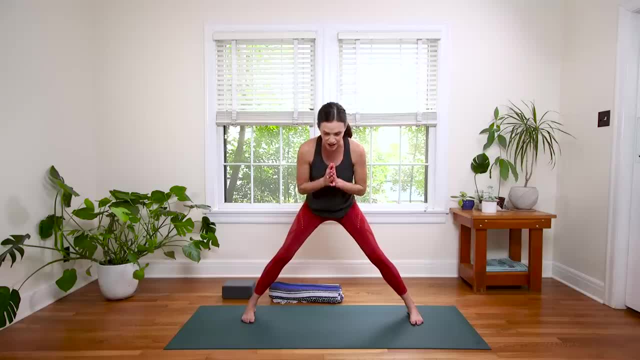 So the goal is to kind of challenge you to keep the inner thigh engaged here, pressing into the outer edges of the feet, creating stability and strength around the knee, Breathing deep, And then you're gonna bend the knees and really find that connection from the ground up. 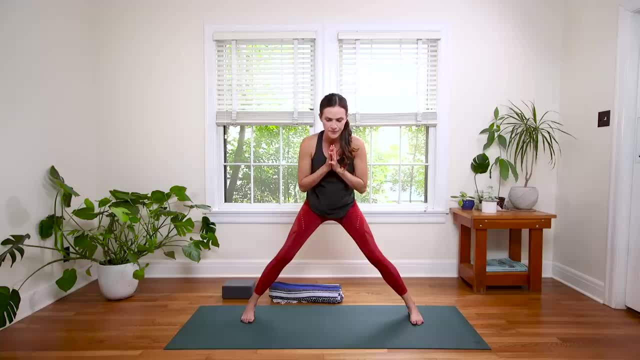 So work from the ground up to rise up, nice and slow. And if the legs are tired here and you feel weak, no, the legs are tired because you're waking up not just the muscular body, but the energetic body as well. All right. 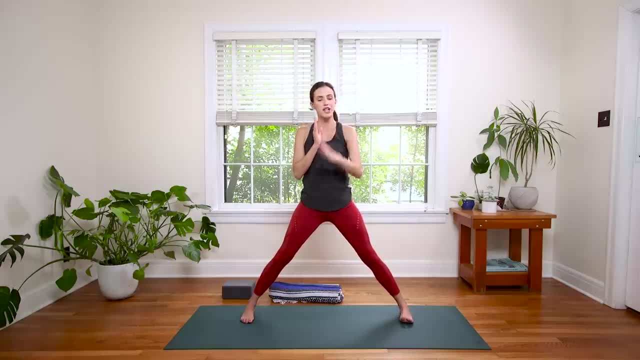 Turn the left toes in very gently, Keep the left inner thigh engaged, In fact, bring your left hand to your left inner thigh and just give it a pat to kind of feel: oh yeah, what does it take to engage that muscle? All right, 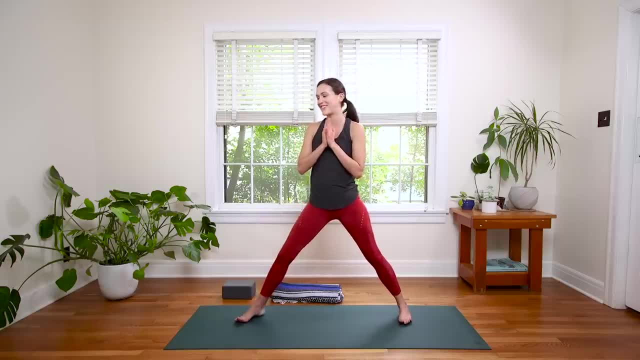 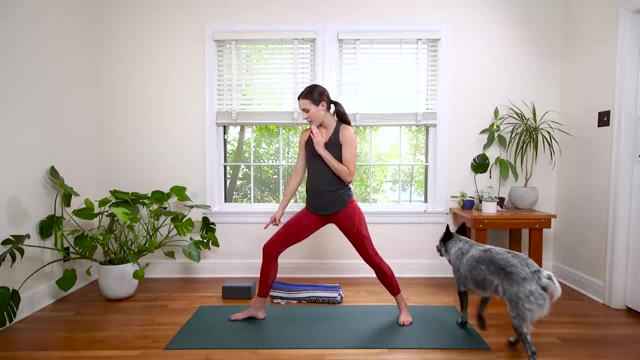 And then, after you've done that for like an awkward amount of time, then you can stop and turn the right toes forward and then we're gonna, nice and slow, we're gonna track the knee over the middle toe. Okay, so open up here. 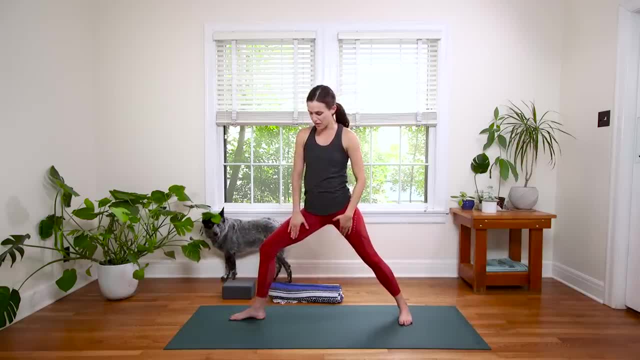 and now we're engaging both inner thighs. Give them both a pat Beautiful, Then we'll come to Warrior II. So we're hugging that right femur in. We're making sure we can always see that big toe. We're engaging both inner thighs. 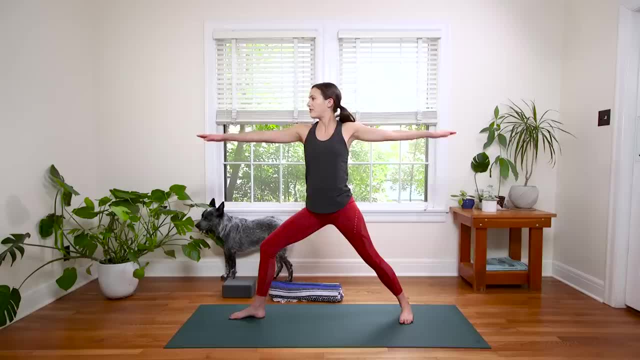 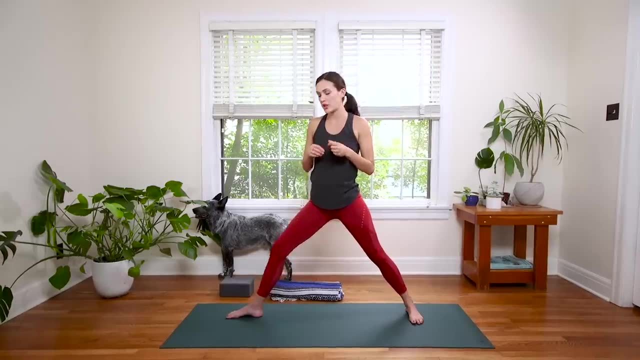 finding that inner lift through the inner groin. Benji, you're being funny today And then we'll come into Warrior II. So I find, for people who are trying to build stability and to strengthen the knees, going that super wide stance isn't really helpful. 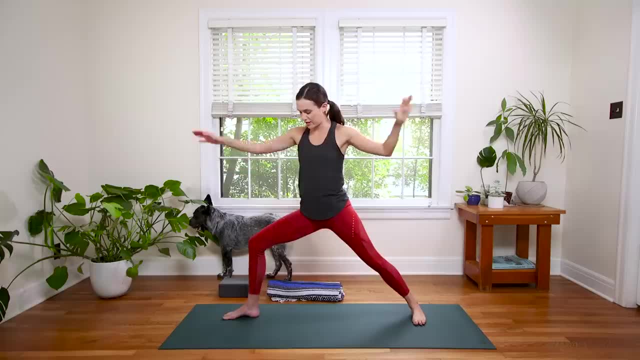 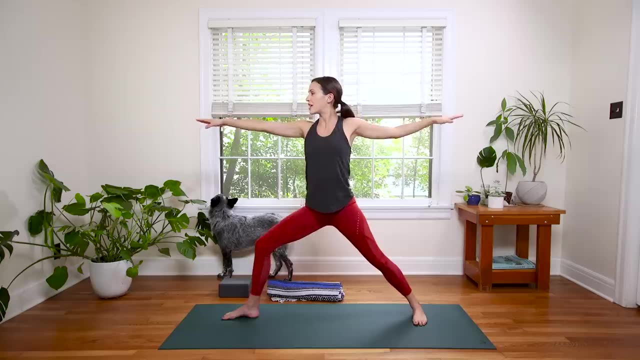 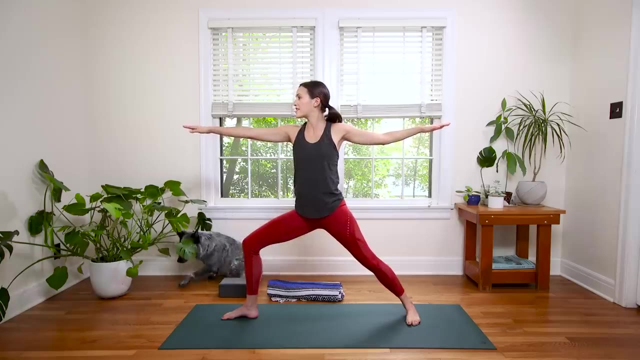 You can work your way there. So notice, my stance is a bit short today, Making sure I can see that front big toe, Left toes are turned in. We're gonna breathe here. Relax the shoulders And just inquire. Strengthen the legs. 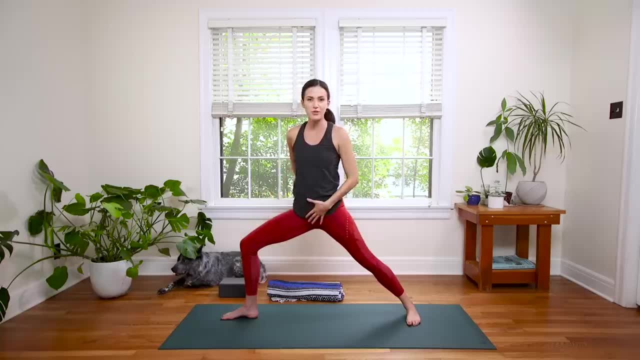 We're here for five: Front knee over front ankle. Four lengthen tailbone down Hips up three, Two, one. Then take the right fingertips up and over Peaceful Warrior Press into the outer edges of both feet. 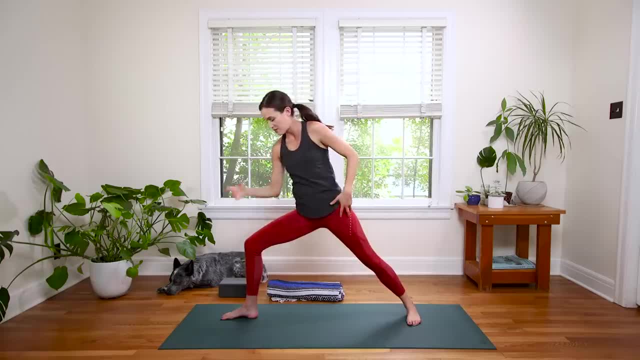 Inhale, lift your chest And then exhale Extended Side Angle. Keep hugging it in, Hugging the right thighbone in, You're gonna send the right fingertips- excuse me, left fingertips- to the sky And right elbow can come onto that. 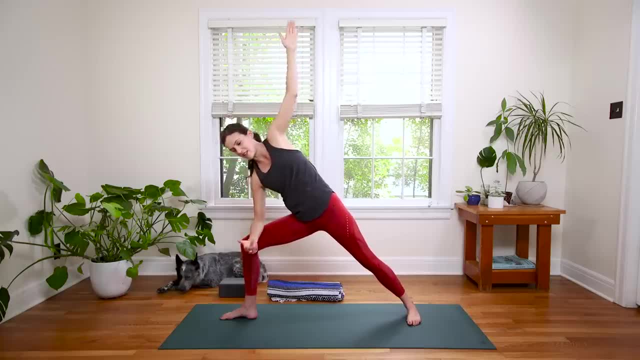 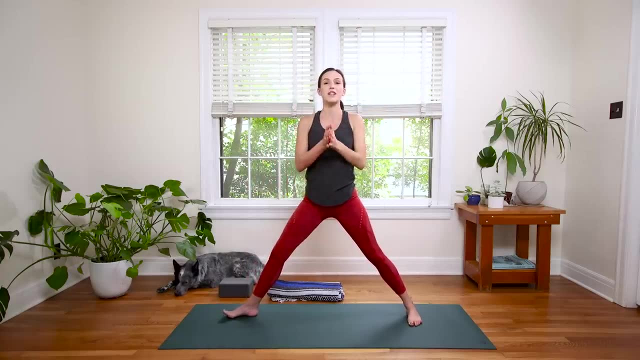 But you're wanting to keep your core strength, not press into that knee. What good does that do? Awesome. then left fingertips reach up towards the sky, Bring you back up to center. Palms come together at the heart. Toes turn facing forward again. 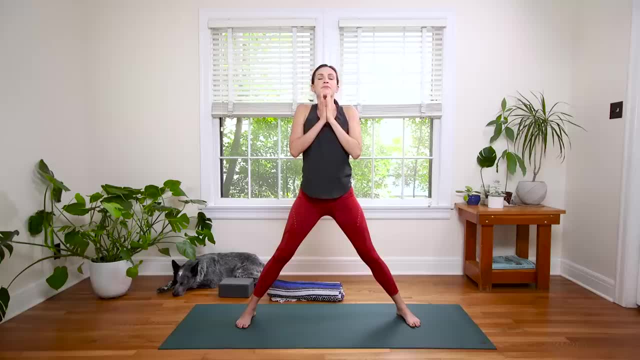 We take a deep breath in. Lengthen tailbone down, Heart lifts up And exhale. relax the shoulders- Awesome. Turn the right toes in, Press into the outer edge of that right foot, Engage the right inner thigh. So the power of these Warrior Postures. 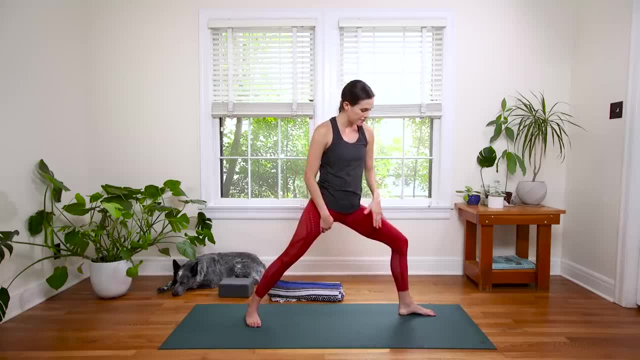 coming from the back leg And we turn the left toes out, Front knee over front ankle, Lengthen tailbone down, Hip points up- Make sure you can see that front big toe- And then really engage the inner thighs so much that they're drawing zipping up and in. 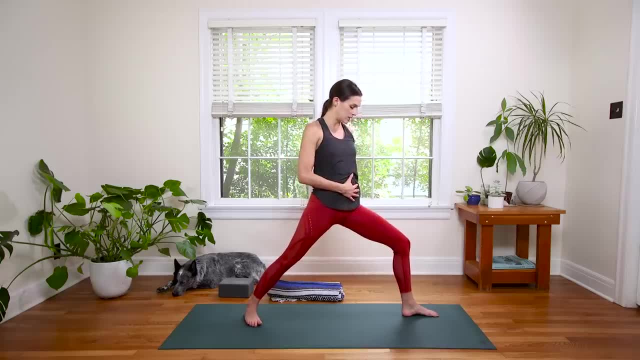 Lengthening tailbone down. Let's take a couple moments to feel it out here And when you're ready, find your arms. Virabhadrasana II, And again today, shorter stance If you don't have weak knees or, excuse me, sensitive knees. 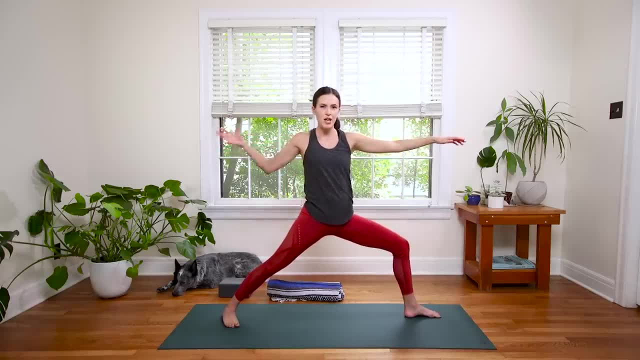 then you can go wide. But I'm just saying, I'm just trying to pull it back a little for those who are wanting to continue to deepen their practice Find that engagement. So there's no point in hitting the pose or the mark if it's not doing the body good. 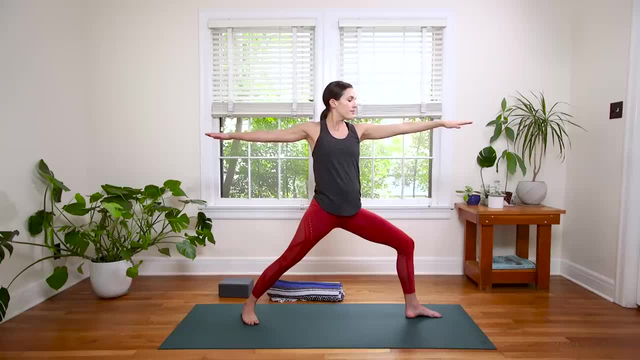 And take one more breath here. Five, four, three, two, one Left fingertips reach forward, up and back. Peaceful Warrior, Try to keep this length through the right side body all the way up. Front knee stays bent Strong and engaged through the inner thigh, inner groin. 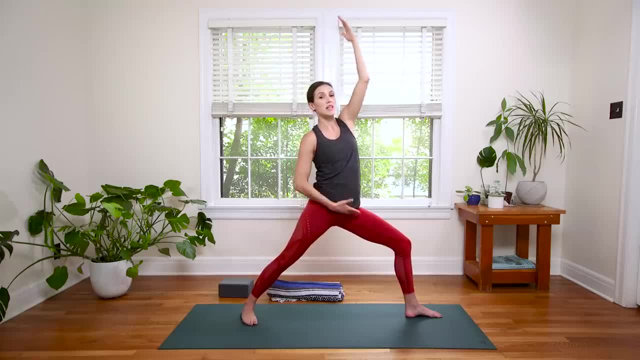 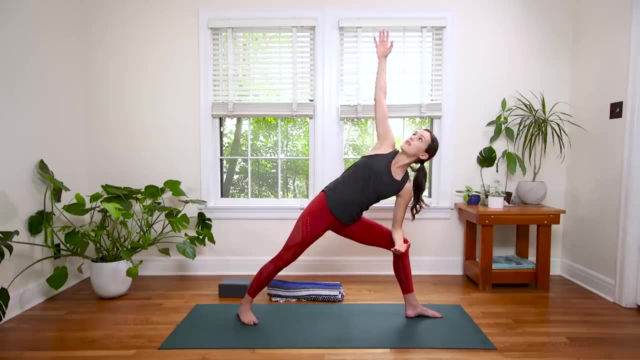 Take a big stretch, big breath, And then here we go, lifting up. Keep the lift up all the way so we're not crashing into the joints. Extended side angle: Right fingertips to the sky this time, And then just notice the awareness. 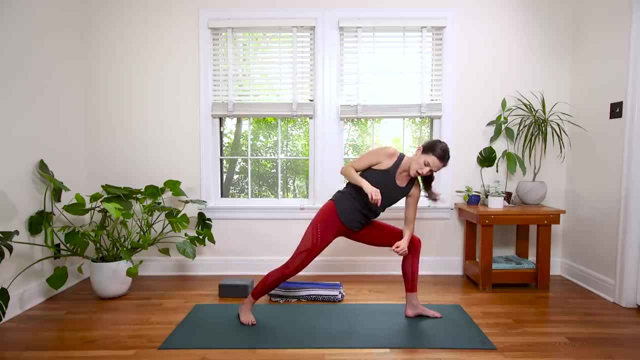 Since this whole video is about being kind to the knees, notice if you're kind of crashing down into your knees, Or if you can draw strength from the earth. I mean, this is a warrior sequence, For heaven's sake, So reach for the sky. 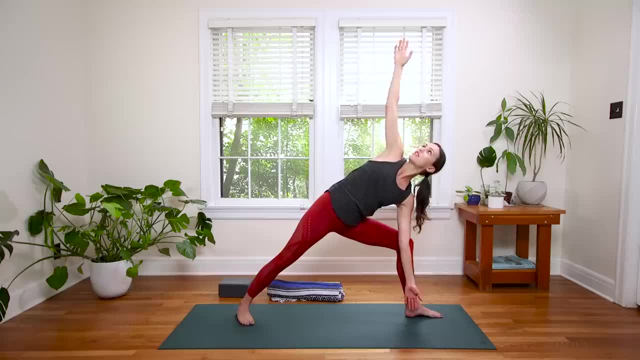 Strong and steady. You won't even need this in time. When you build strength, you'll be able to hover- No extra pressure on the knee, Just strong and stable, And then to come up, reach the right fingertips all the way up to the sky. 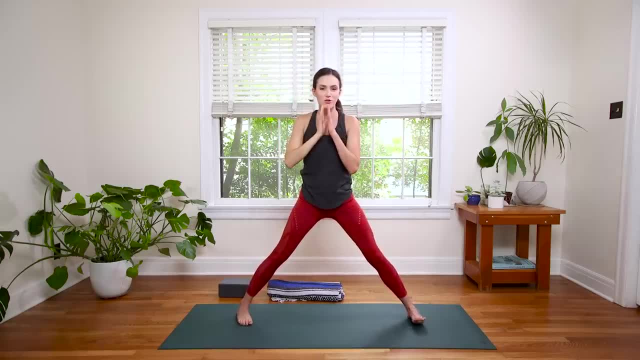 Smile just a little bit And we'll come all the way back. Hands Anjali Mudra at the heart, Toes pointing forward, Deep breath in Exhale. release everything And then you're just gonna step the feet together. 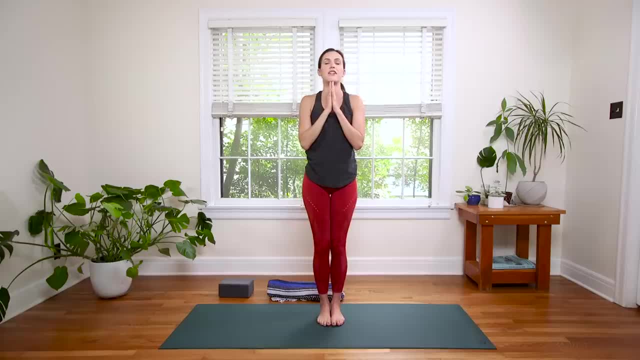 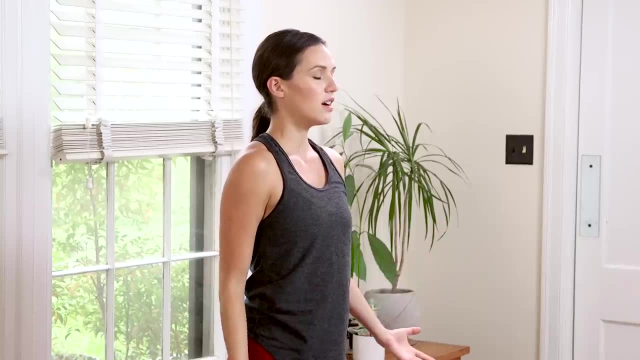 nice and slow. You want it to look down? Feet together, really together, really together, really together. Take a deep breath in Mountain Pose Exhale, release the fingertips down And see if you can zip up the legs here. 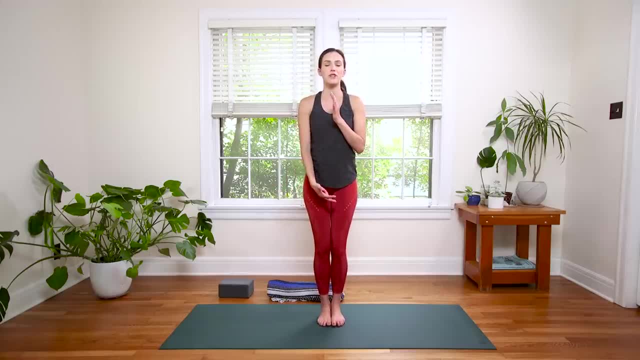 and spread weight evenly through all four corners of the feet, knowing that that information travels up to the knees, to the hips, to the heart, the shoulders and up through the crown. Take a deep breath in, Along, exhale out. 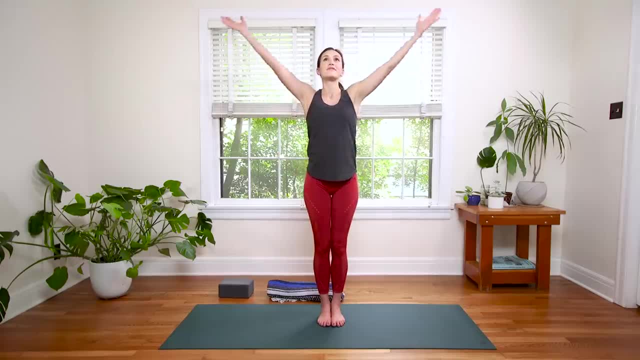 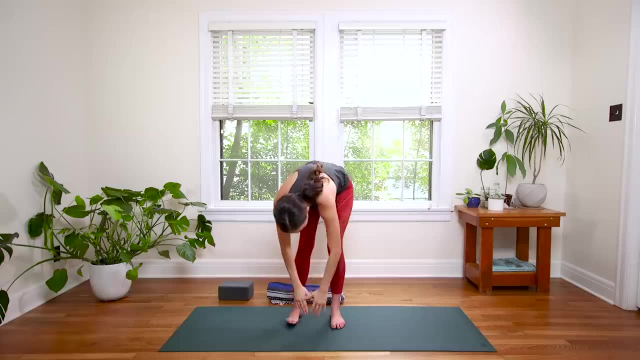 And then inhale to reach for the sky And then exhale slowly all the way down. If you need to step the feet hip width apart here you can bend the knees as generously as you need to And plant the palms. step it back one Plank Pose. 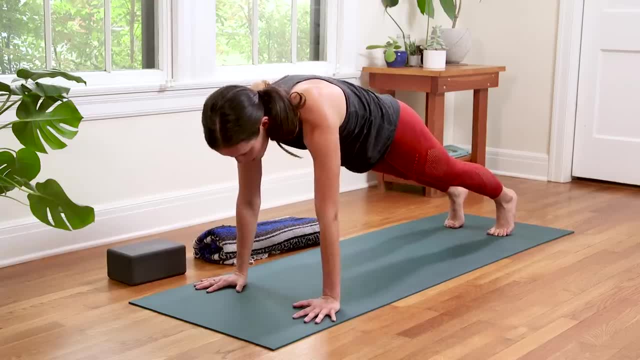 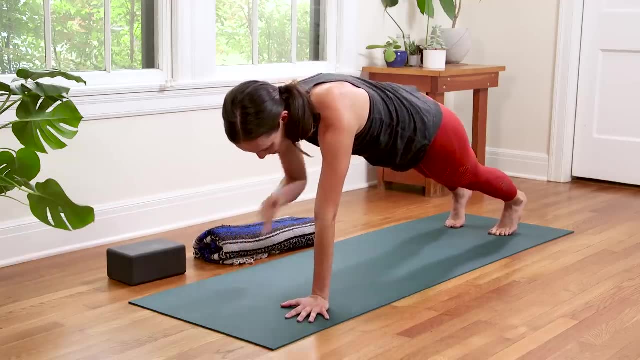 All right in your Plank Pose, reach the heels back, press away from your yoga mat. Try to keep the hips where they are in space and touch the left fingertips to the right shoulder. Then bring the left hand down and touch the right fingertips. 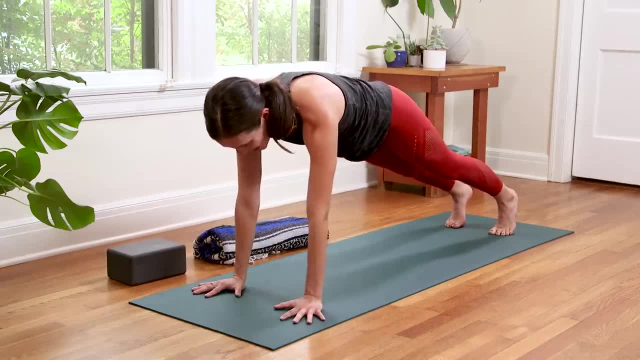 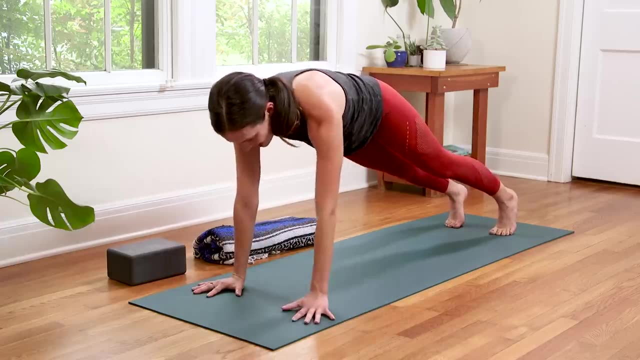 to the left shoulder And now back and forth, gaze straight down. You're gonna try to keep your hips where they are in space- Super core strength in here, Breathing deep, you got it And even it out And then slowly release. 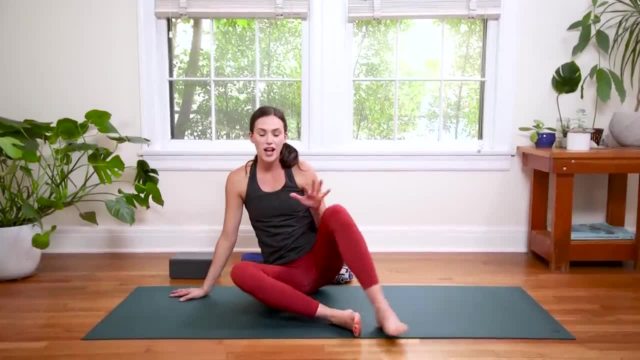 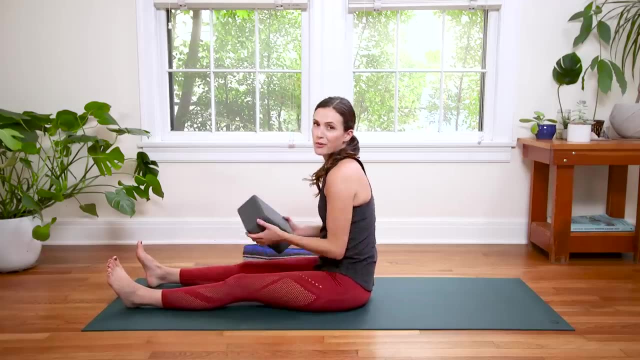 Awesome. you're just gonna come onto your bum, Send the legs out wide, Yay, And if you have a block, you're gonna grab the block now, And then we're all gonna come to lie flat on our back with the feet on the ground. 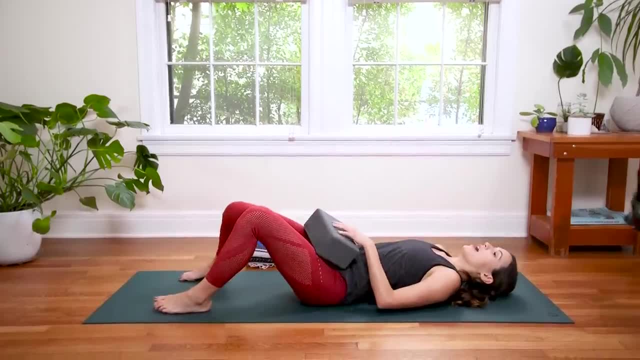 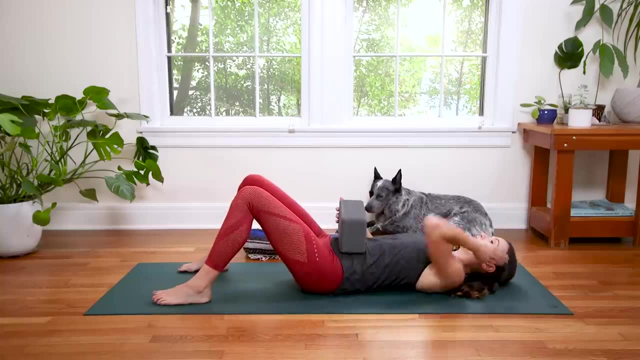 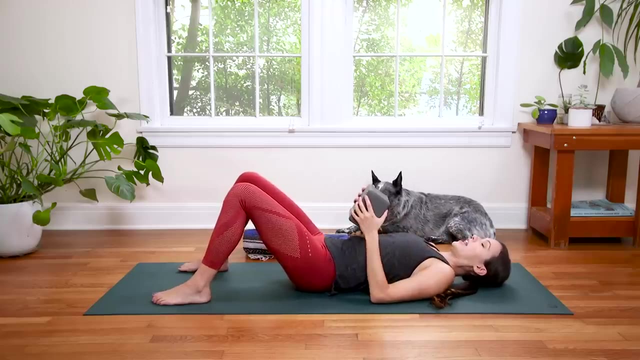 So take your time getting there, Wipe any sweat off your brow, Take a nice big refreshing inhale in through the nose and out through the nose or mouth. So we're ending with a little bridge twist, relax sequence. So the thing about bridge is, if you don't know, 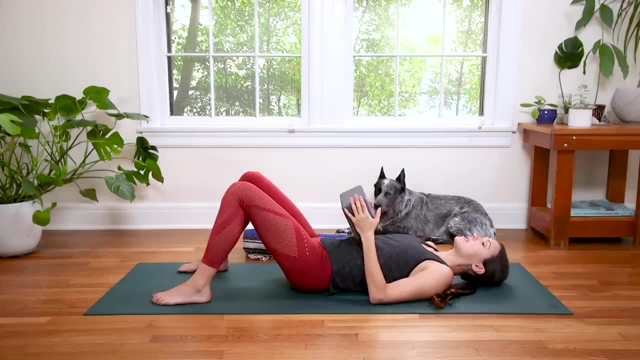 what Satubandhasana, or bridge pose, is. go ahead and watch me the first time, because it's not the type of pose where you wanna look at the video when you're in it. It can cause a little bit of harm to the spine. 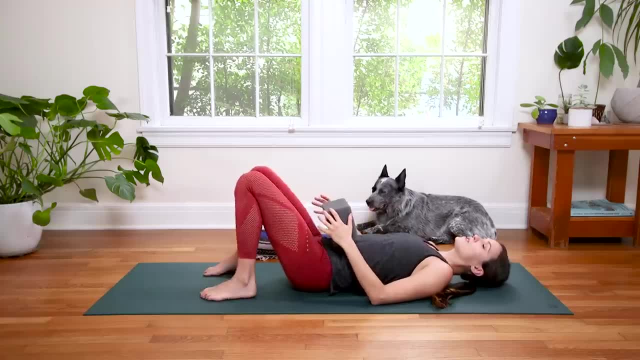 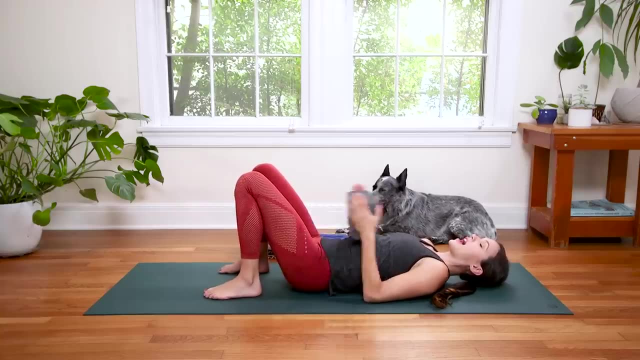 and that's the opposite of what we're trying to do here, y'all. So bring the heels up. fingertips are gonna reach down and this is a nice little marker: heels to the fingers And if you have a block or something that you can bring between your legs, 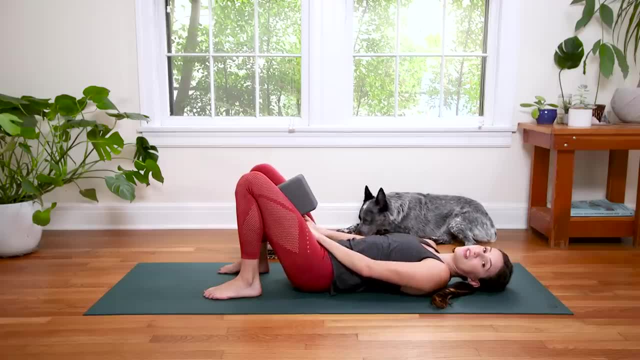 then you're gonna go ahead and use it today so you can squeeze and feel that inner thigh engaging once again And again. you can practice this today or once a week, but remember to take these things with you into, oh, other practices. this is for everybody. 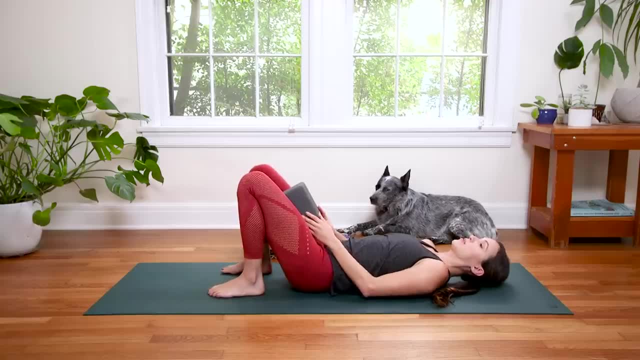 So the knees aren't splaying wide when I have the block. It's nice to get a little reminder, but if you don't have the block put in a little imaginary block in between your thighs. And then- so important- a lot of joint issues. 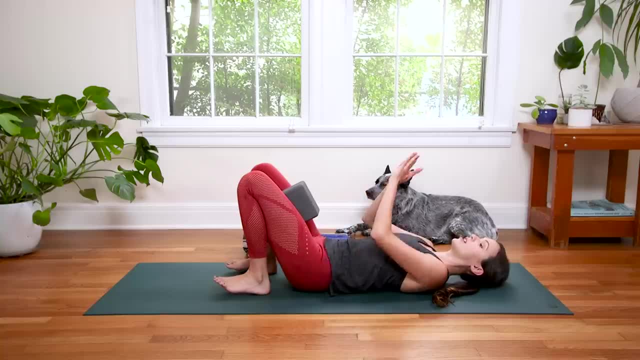 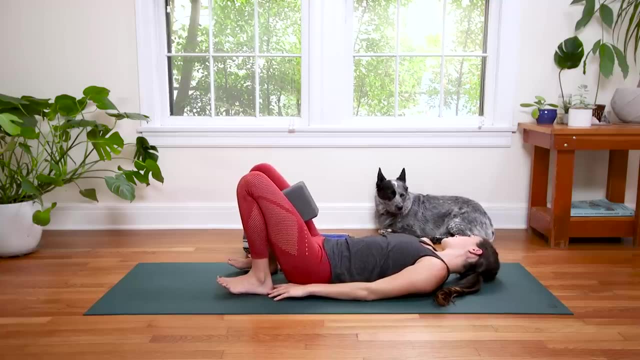 you know they stem from the foundation of whatever it is. So the hands for the wrists, the feet for the ankles and the knees, So find that foot to earth connection, Baddha Bandha, And really root down through the ball joint. 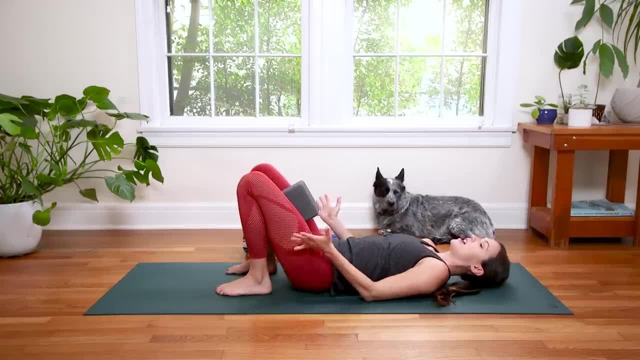 and that big toe ball joint of the pinky toe and the back two corners of the heels. Then squeeze your block, Use your hands to guide you. We're gonna scoop the tailbone up and nice and slow from the feet. So often we think about hips lifting up. 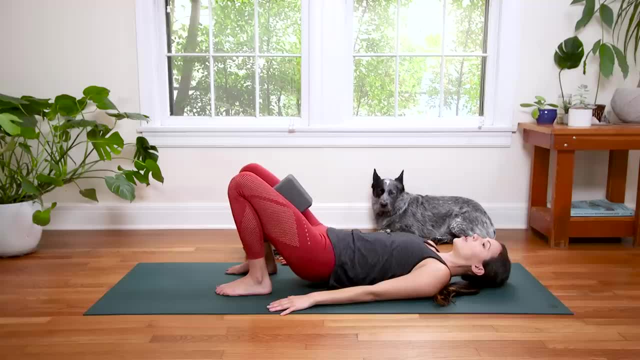 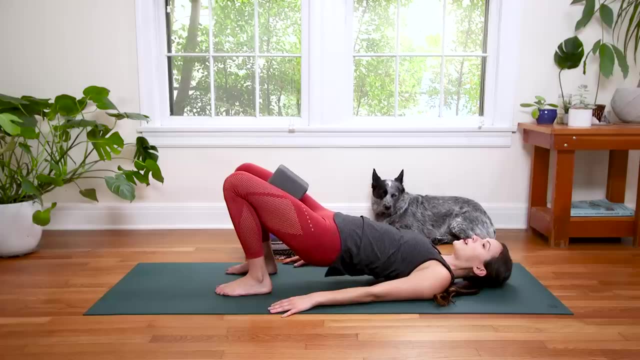 Really pay attention to your feet, Pressing your feet so much so that the hips start to lift up And we're pressing evenly through all four corners of the feet- and really pay attention to the nuance there. We tend to forget about the feet and just really try to get it. 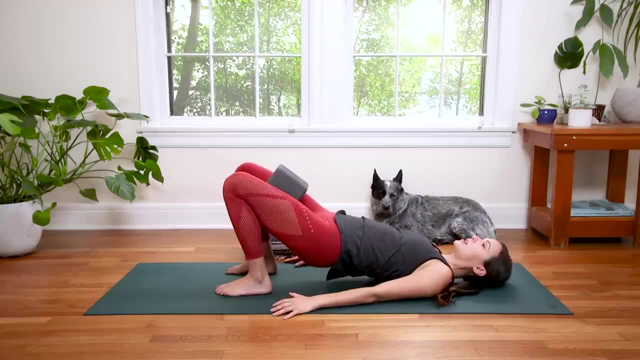 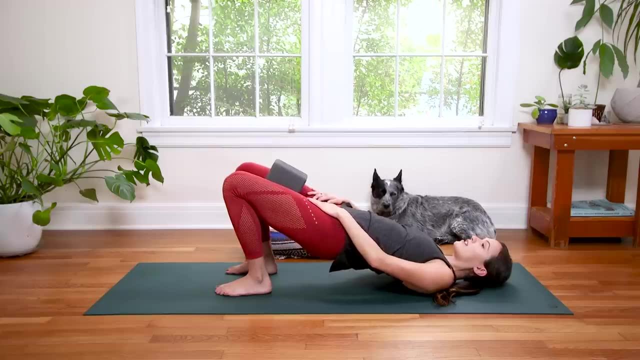 in the right place We try to get to this bind. So really lift up, feel the nuance and feel the block as you lift the hips, the inner thighs engaged to stabilize, to strengthen. Then send the shin bones forward, Hug the femur in, lift the hip points up high. 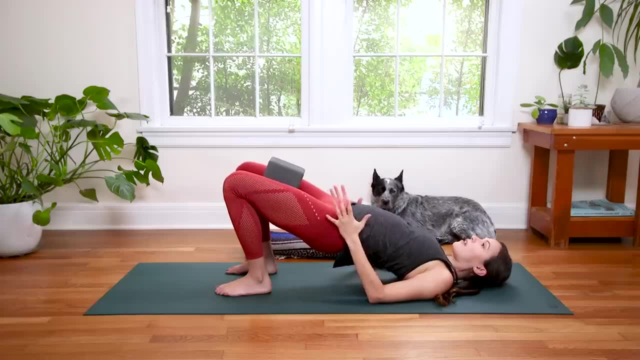 and see if you can do this- here's the kicker- without clenching the glutes. See if you can engage the inner thigh. Obviously, we're toning the quad without clenching the glutes. Press the palms into the earth, inhale. 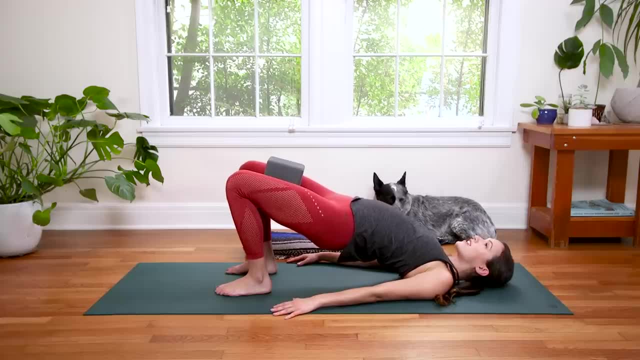 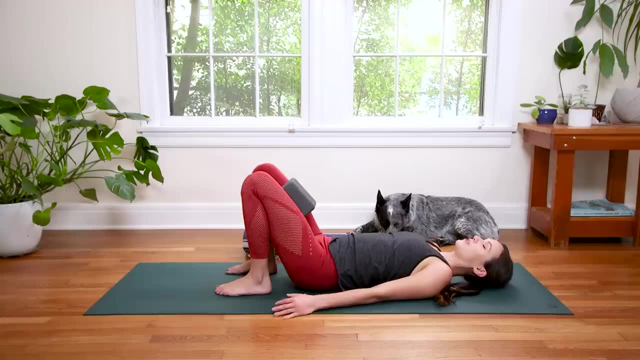 And then exhale, lift your chest to your chin and your chin to the sky, should feel awesome And release everything down. Awesome, take a little break, sigh it out, Close your eyes And one more time. I'm gonna talk less. 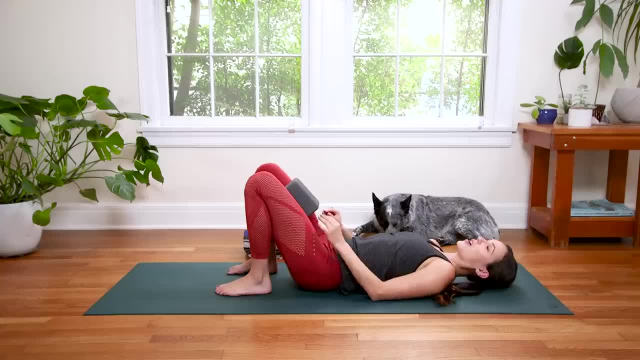 but I want you to really try to find where the muscles turn on, See if you can soften through the glutes and this time, if you wanna take the bind you can So strong. focus on the feet. here we go, Inhale, lifting you up. 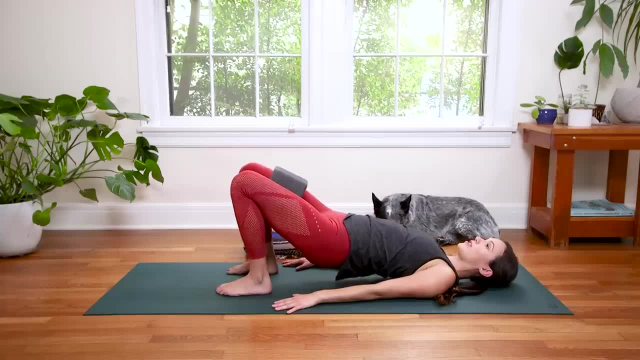 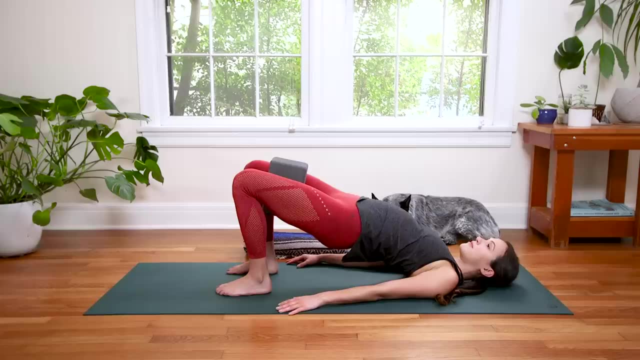 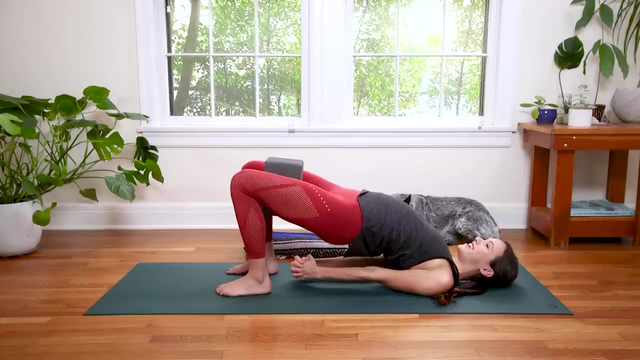 Listen to the sound of your breath. squeeze your block, or your imaginary block Shins forward. hug the femur in, lift the hip points up, high Chest to chin, chin to the sky. Maybe you walk the shoulder blades underneath, Engage the inner thigh. 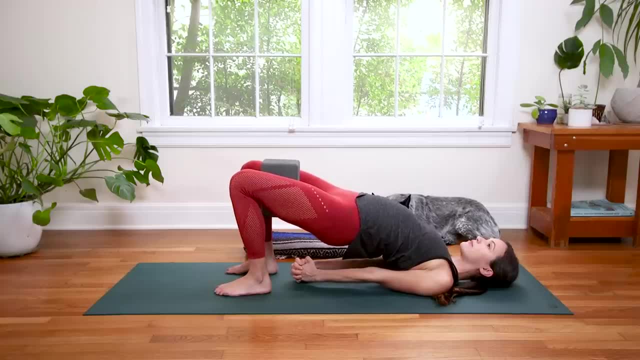 Exhale inhale exhale exhale exhale exhale exhale, Exhale, inhale, exhale, exhale, exhale, exhale, exhale, exhale, Exhale, inhale, inhale, exhale, exhale, exhale, exhale exhale. 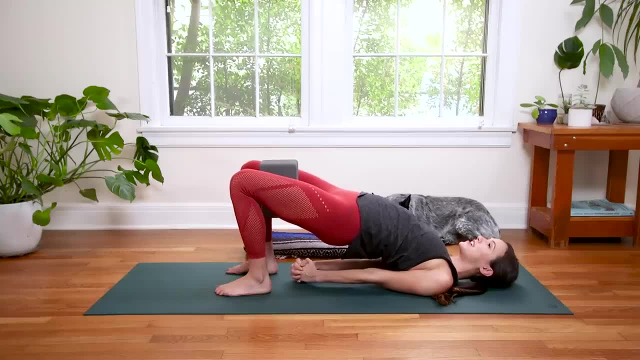 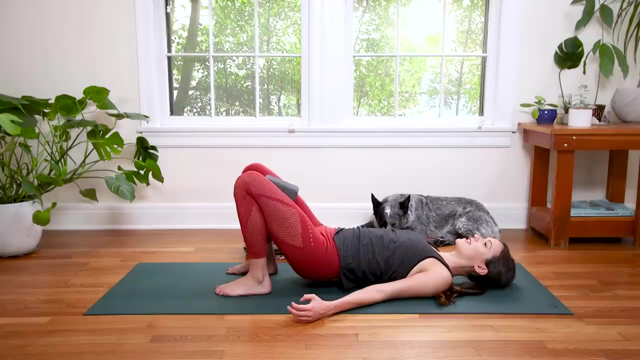 Keep uncovering, keep adding to subtracting, Pay attention again to the nuance And then slowly release the bind, if you have it, and bring it down nice and slow and with control. So another thing I will add is: a lot of times things happen with the knees. 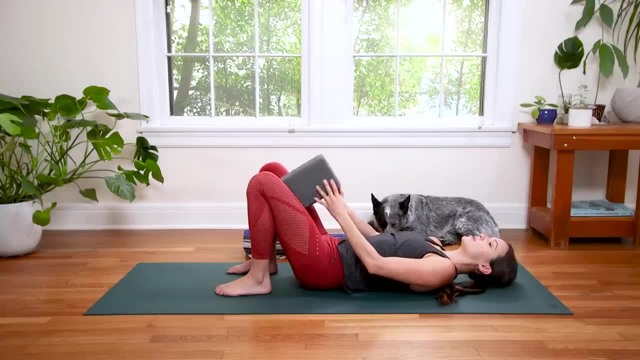 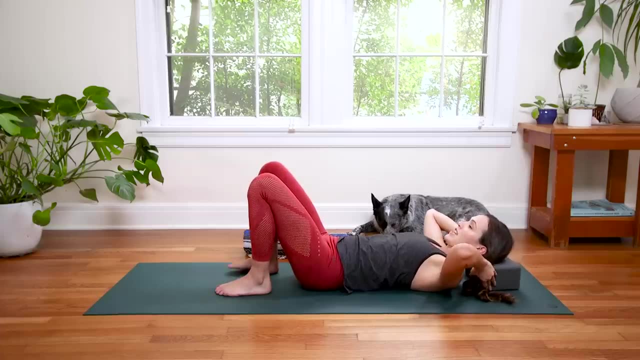 in between poses, not during, but the consciousness in between. Take your block. you're gonna bring it to the side, or you can bring it to your head for a pillow. Then we're gonna come to that nice Supta Baddha Konasana again. 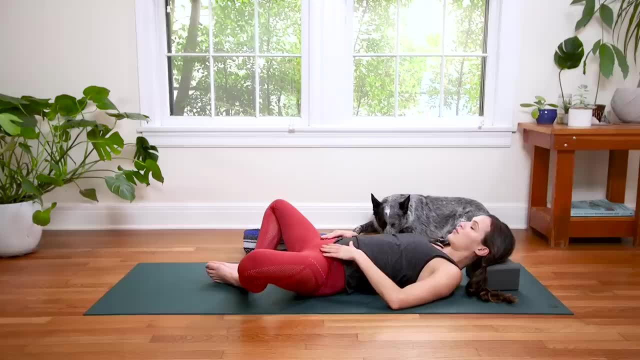 So, knees wide, soles of the feet together, hands on the hips, breathe deep, Let everything go. We're almost done here. so really activate the breath, take your vitamins. Nice control of your breath, slowing it down, Can completely change your day and maybe your life. 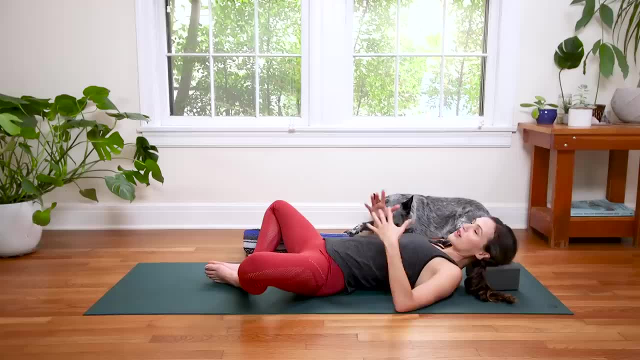 So use this time with me and with everyone else who's practicing this around the world, to just check in before we get up off the mat. And we'll do that by breathing deep. Use your hands to slowly guide the thighs, the knees together.